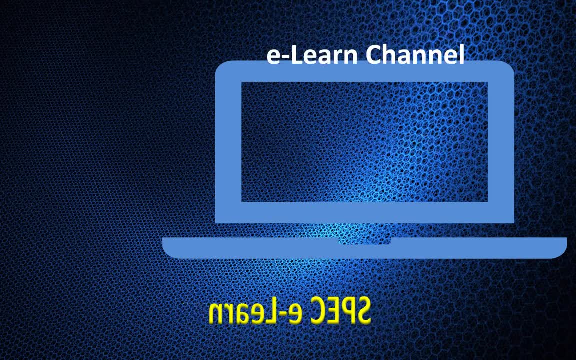 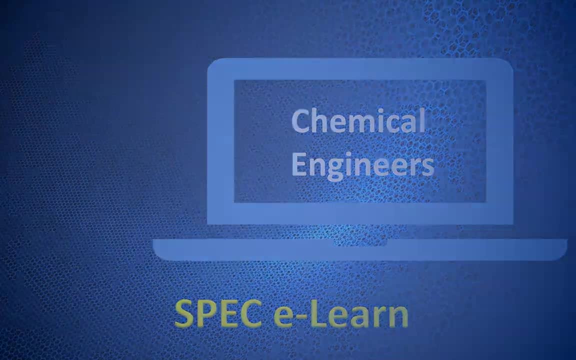 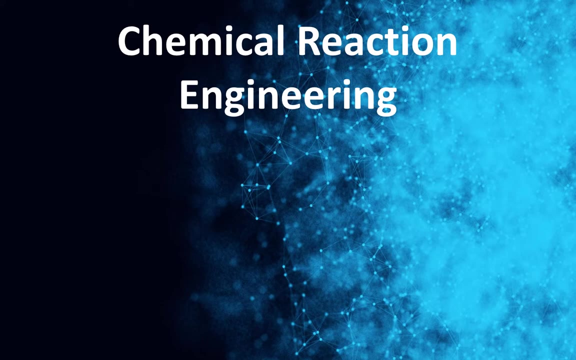 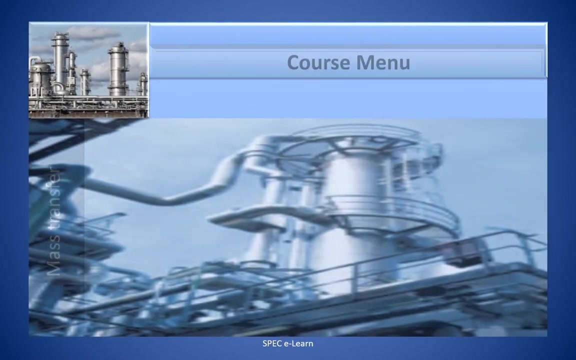 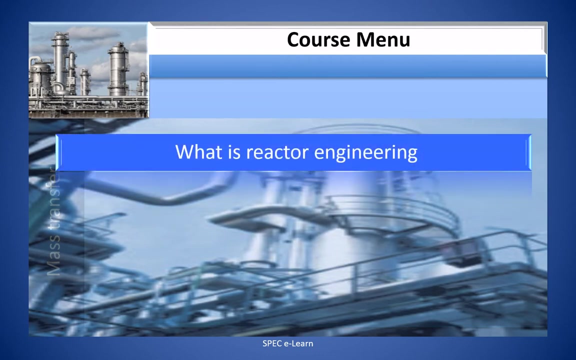 Hello everyone, welcome to SPECT eLearn, the online learning channel dedicated to chemical engineers. Chemical Reaction Engineering. Part 5: Reactor Engineering. This video focuses on reactor engineering related to catalytic reactors. In this video, you will learn what is reactor engineering, what are the important parameters to be considered in selecting and designing reactors. 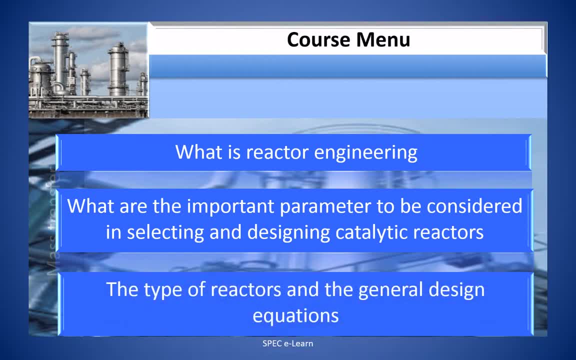 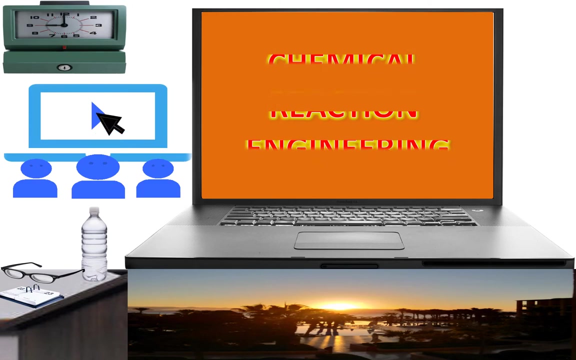 the type of reactors and the general structure of reactors. I would appreciate if you subscribe to the channel, which is striving hard to deliver valuable knowledge content for your career progress. So subscribe now, before you forget. Reactor engineering refers to design and development of reactor hardware for meeting the desired reactor performance. 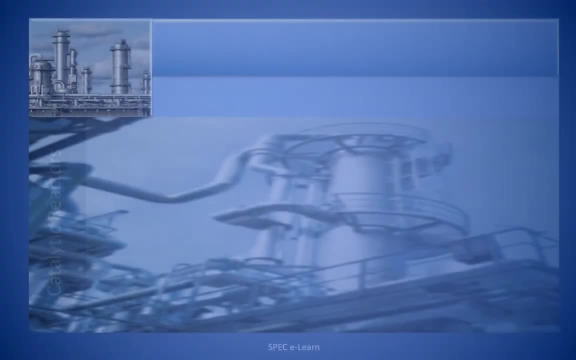 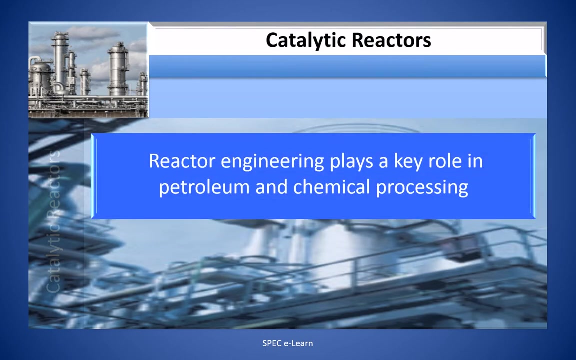 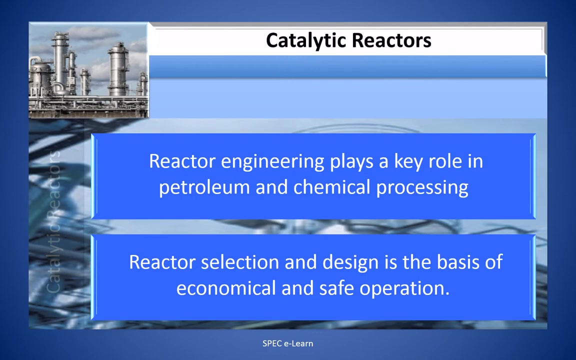 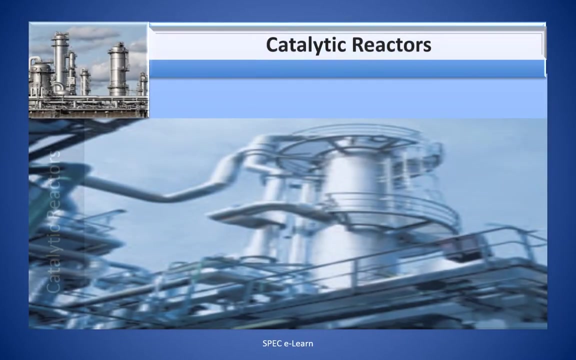 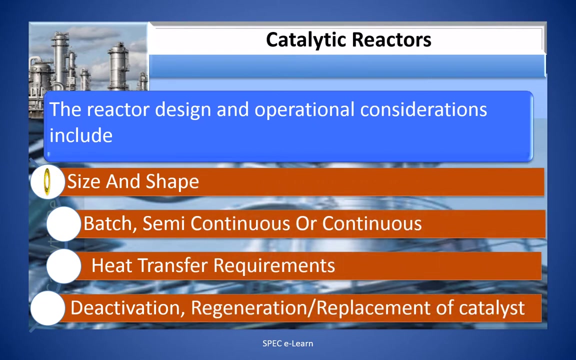 Reactor engineering plays a key role in petroleum and chemical processing. Reactor selection and design is the basis of economical and safe operation. Reactor design and operational considerations include Design and operational considerations include size and shape of the reactor. batch semi-continuous. 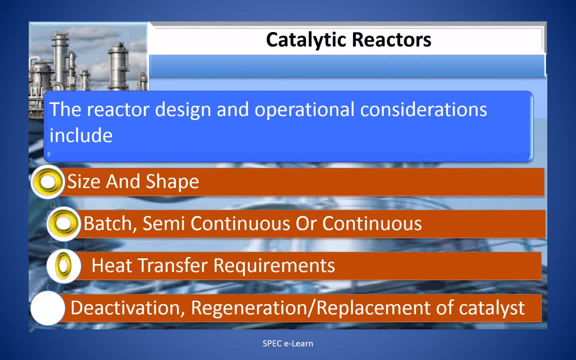 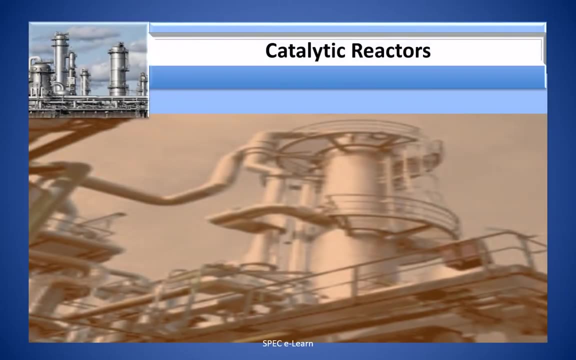 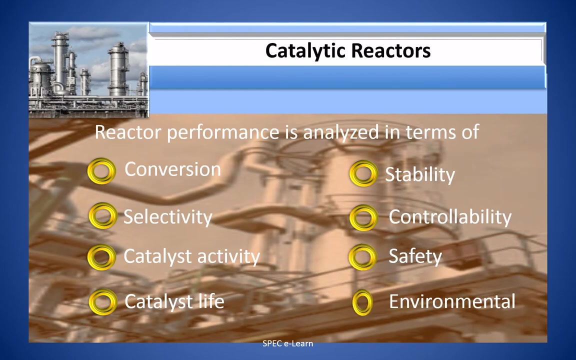 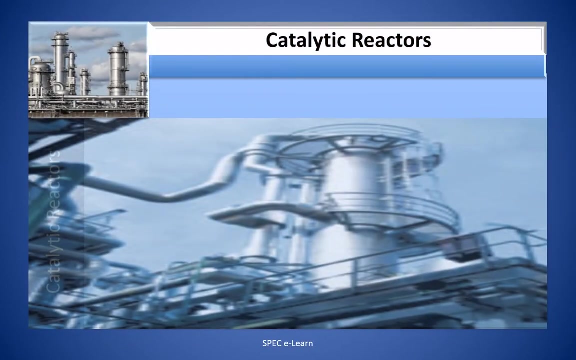 and continuous heat transfer requirements, deactivation, regeneration or replacement of catalyst. The reactor performance is analyzed in terms of conversion selectivity, catalyst activity, catalyst life stability, controllability, safety and environmental issues. These performance parameters are important design considerations. 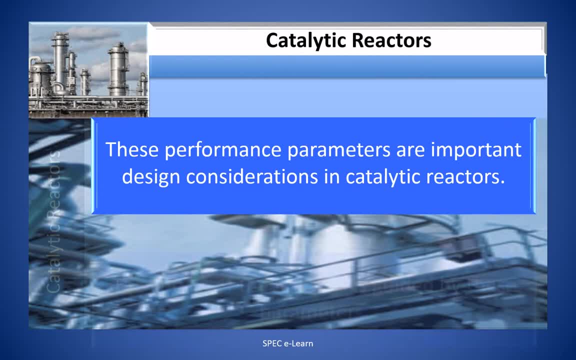 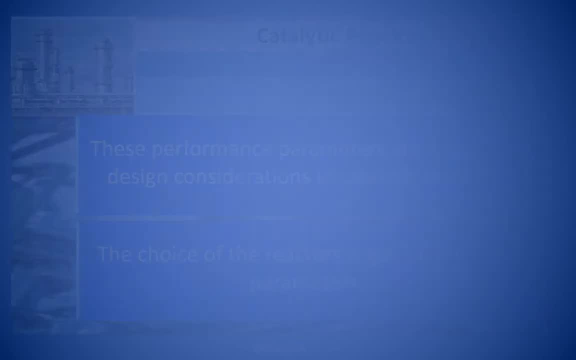 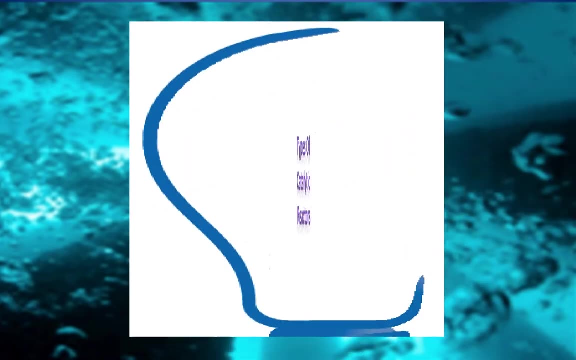 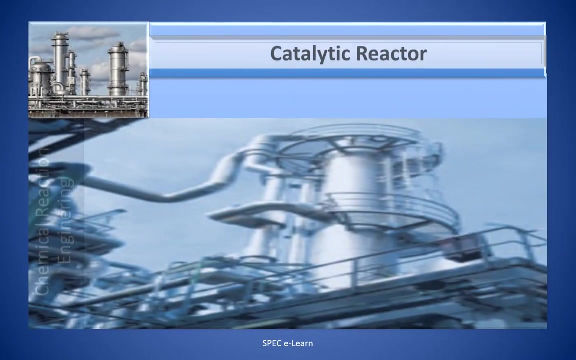 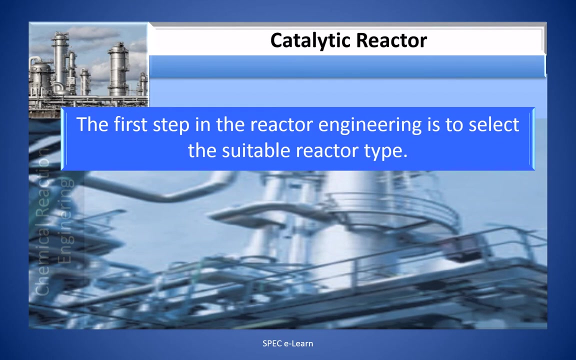 The choice of the reactors is guided by these parameters. Having understood the base of design of catalytic reactors, let us now move on to have a look at the type of catalytic reactors. The first step in the reactor engineering is to select the suitable reactor type. 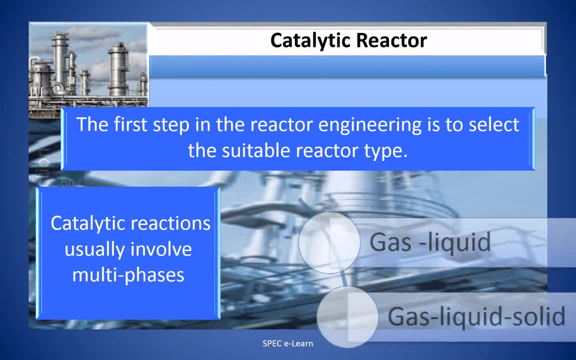 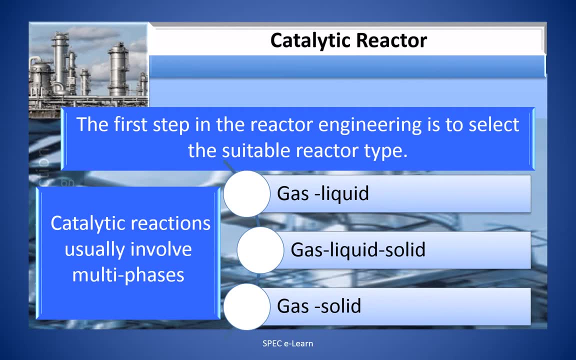 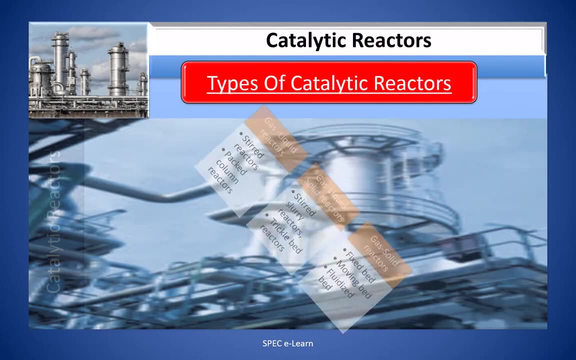 Catalytic reactions usually involve multi-phases: Gas-liquid, gas-liquid and solid. gas and solid Gas-liquid reactors are the most common type of catalytic reactors. The most common type of catalytic reactors are the gas-liquid and the solid. 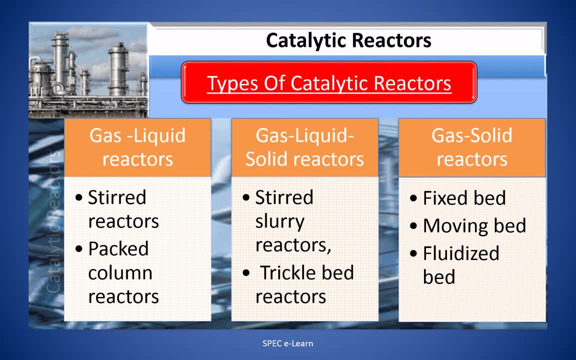 The most common type of catalytic reactors are the gas-liquid and the solid Gas. solid reactors include stirred reactors and particle- stalking reactors, and the gas and solid reactors include stirred slurry reactors and trickle- bed reactors. Gas solid reactors include fixed-bed reactors, moving-bed reactors, fluidized-bed reactors. 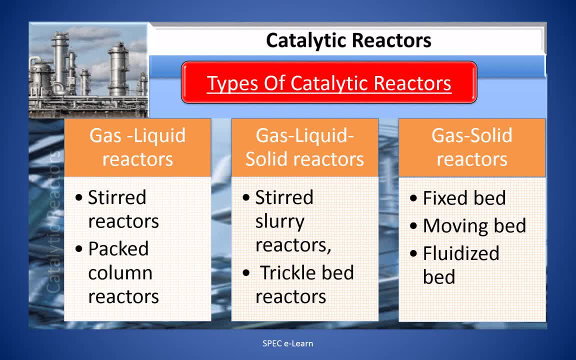 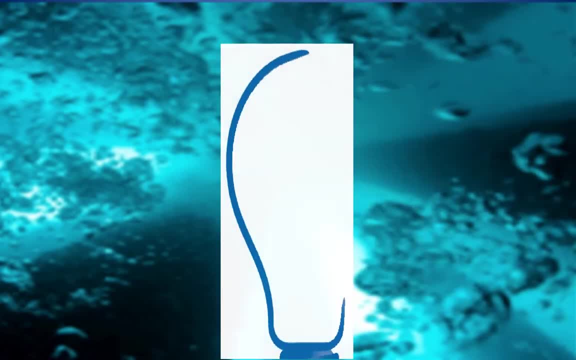 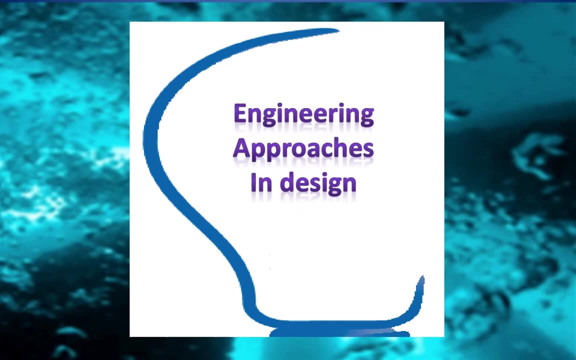 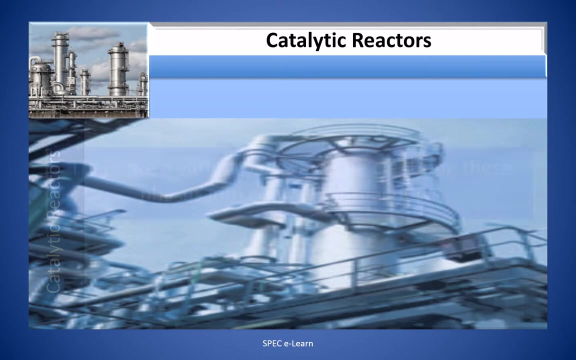 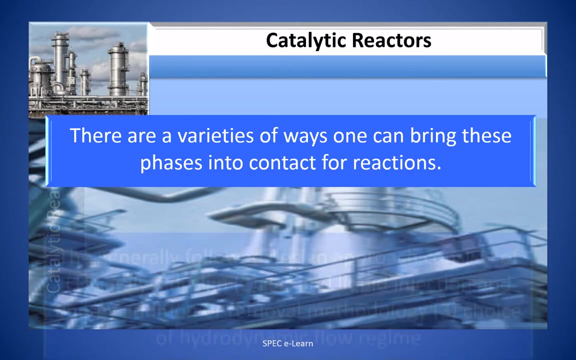 Gas solid reactors involve distillers and carbon deposits and are in two facets. Now let us look at the engineering approaches for these reactors. There are a variety of ways one can bring these phases into contact. for reactions, The generally followed design approach consists of: 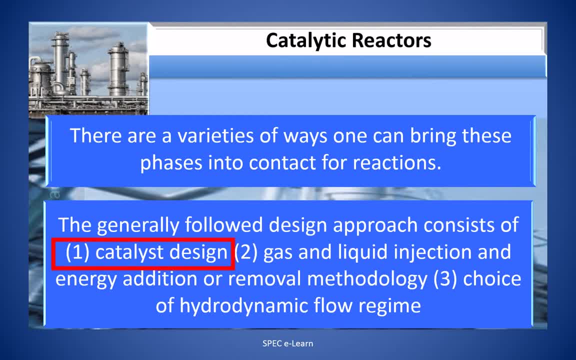 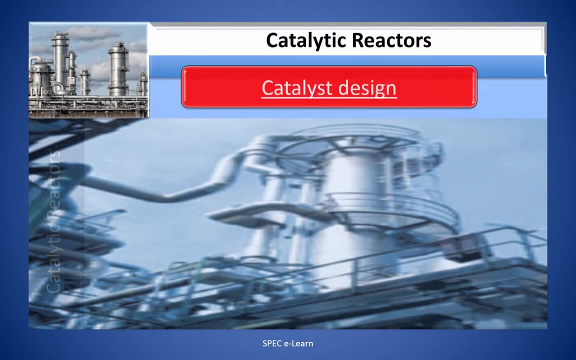 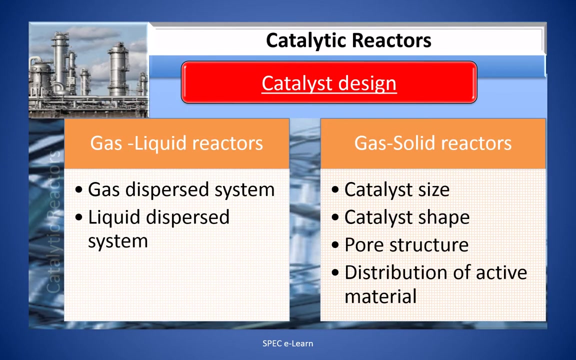 1. Catalyst design. 2. Gas and liquid injection and energy addition or removal methodology. 3. Choice of hydrodynamic flow regime. Let us look at these design strategies one by one: 1. Catalyst design. 2. Gas-liquid reactors- You can have a gas-dispersed system or liquid-dispersed system. 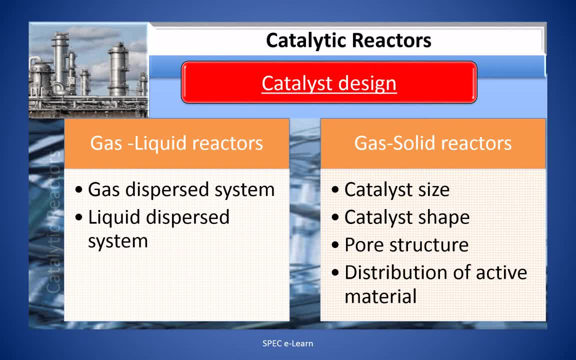 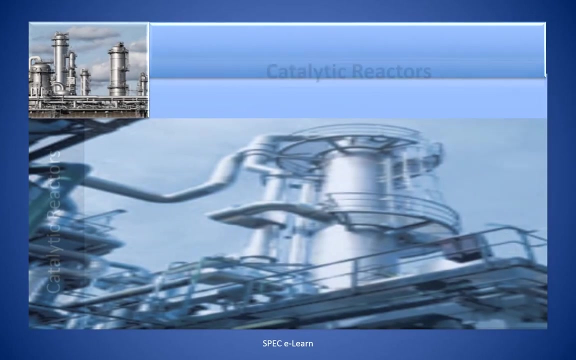 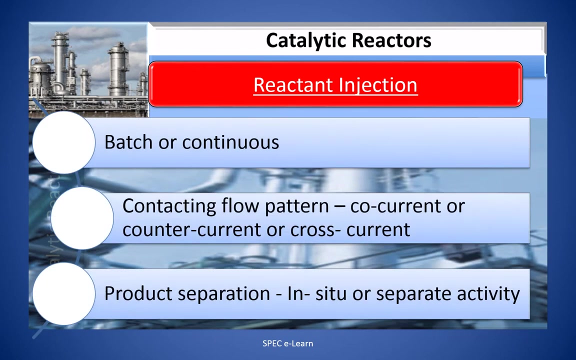 3. Gas-solid reactors. The important approaches are: 1. Catalyst size, 2. Catalyst shape. 3. Post structure of the catalyst. 4. The distribution of the active material in the catalyst. Next is the reactant injection strategy. The reactors can be of batch or continuous type. 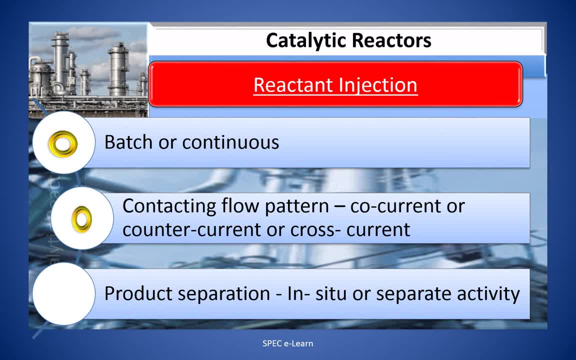 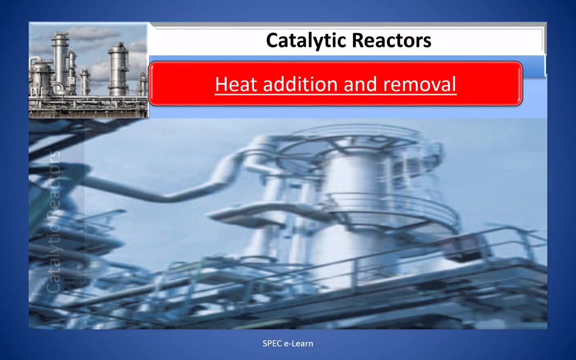 The contacting flow pattern can be of co-current type or counter-current type or cross-current type. The contact flow pattern can be of co-current type or counter-current type or cross-current type. To define the contact flow pattern, the reactor can be of podrige-J might wind cualite causing wear or freeze. 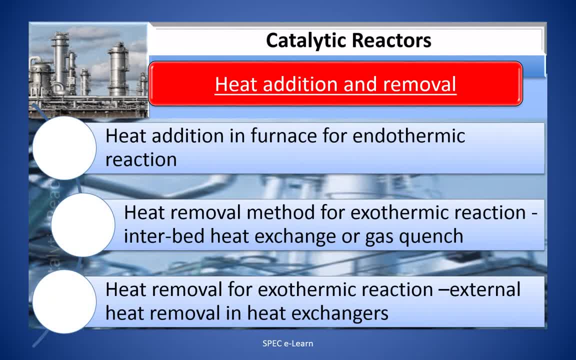 That is the injection rate. may Lang & lets the contact flow rate to be 0.12 or 0.9 or 0.02.. Nanobotany fare: fire heater: Heat removal method for exothermic reaction. It includes intermittent heat exchangers or gas quench, Another method of heat removal. 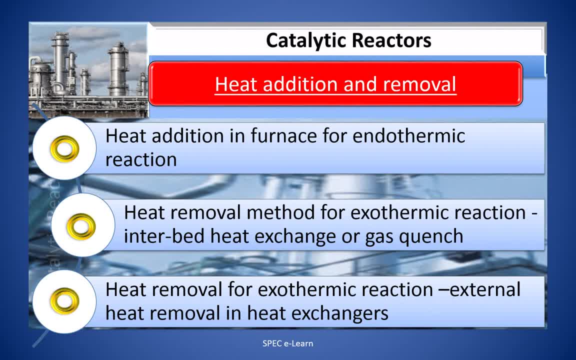 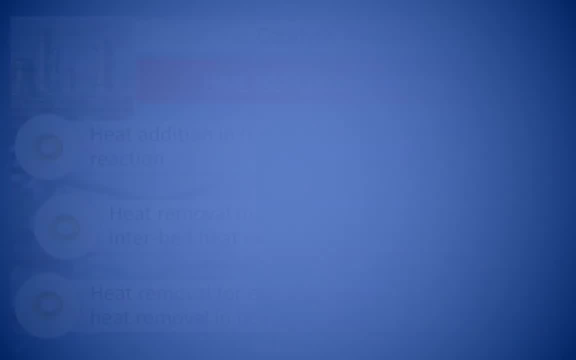 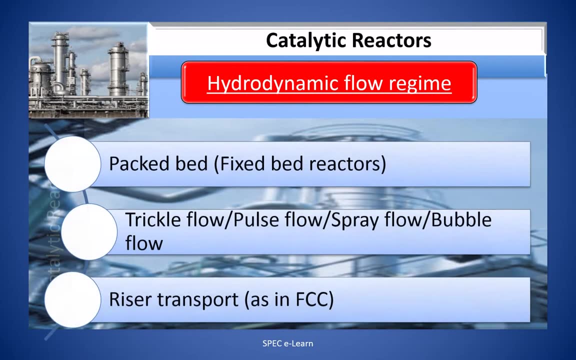 for exothermic reaction is to install external heat exchangers for heat removal. Another strategy to be determined during the design stage is the hydrodynamic flow regime for operation. The hydrodynamic flow regimes include packed bed or fixed bed reactors, trickle flow or pulse flow or spray flow or bubble. 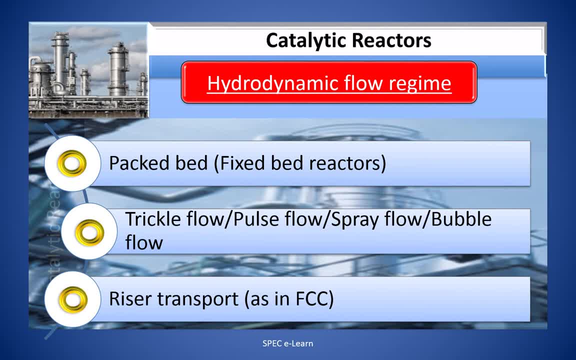 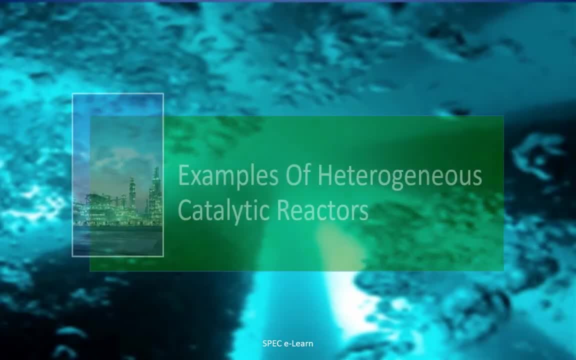 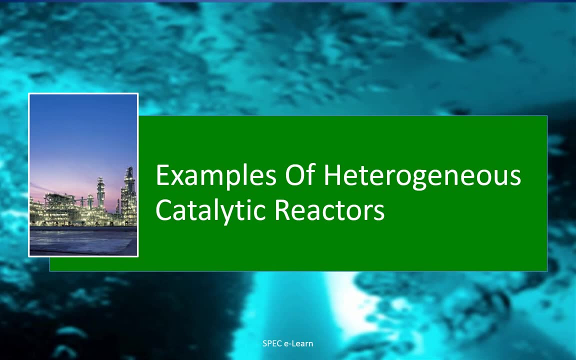 flow and riser transport, As in the case of FCC. Having discussed the design approaches for catalytic reactors, we will now look at some of the examples of real-world reactors where these engineering approaches have been adopted at the design. First, let us look at the examples. 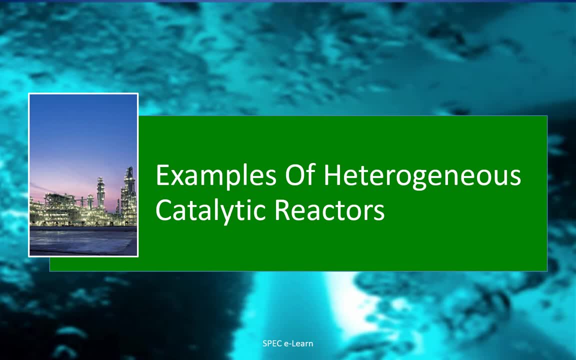 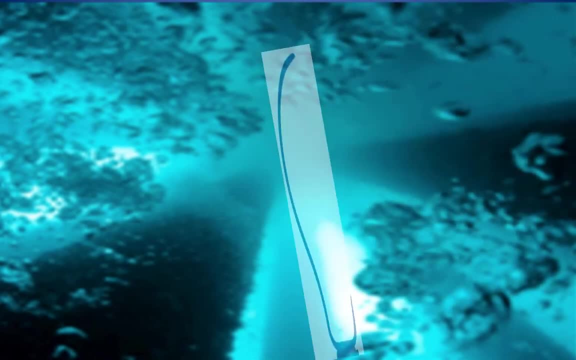 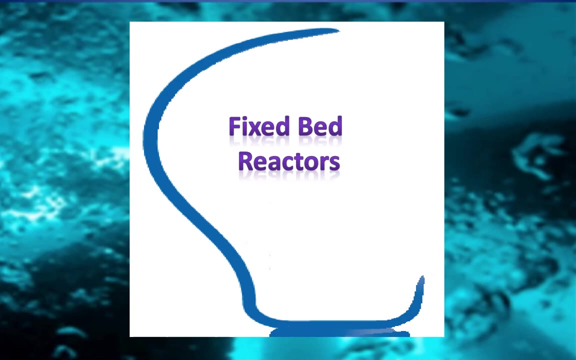 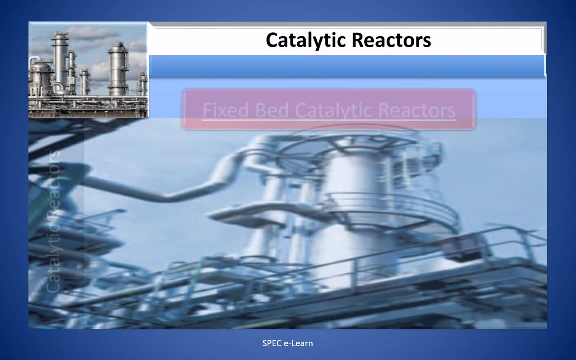 of heterogeneous catalytic reactors. The first among the heterogeneous reactors is fixed bed reactors. Fixed bed catalytic reactors fall into two categories based on their reactor orientation: Vertical fix and parallel Valentine systems. They are typically from one type to another, butny are generally excessively. 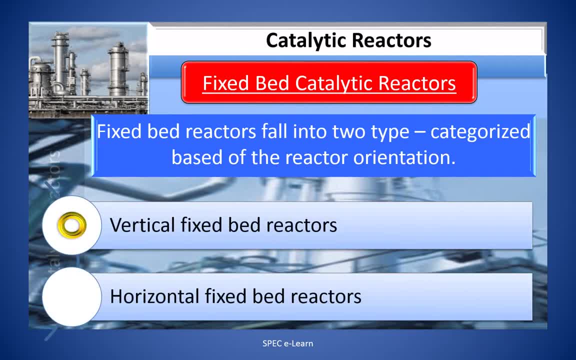 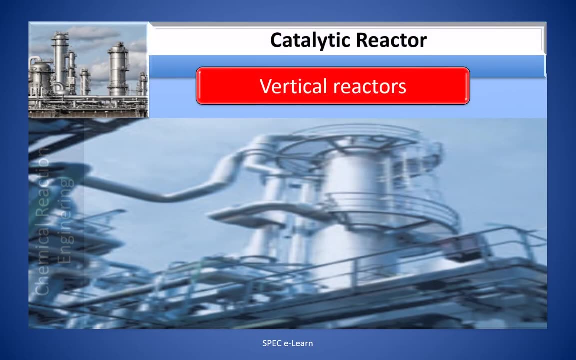 octunacal, Even at an autodidactic rate. we consider the living and renewable energy and neither are above average at typically getting quite opportunities than our target tavae. None of them consider an autodidactic vertical Fickbert reactors and horizontal Fickbert reactors. 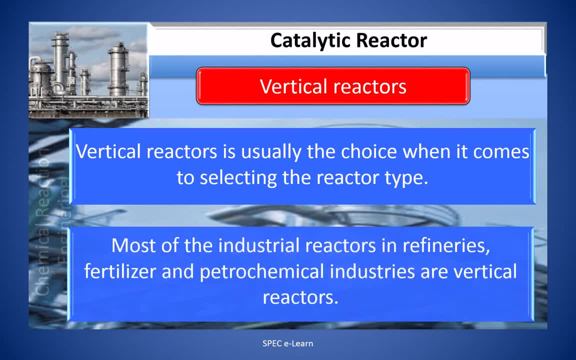 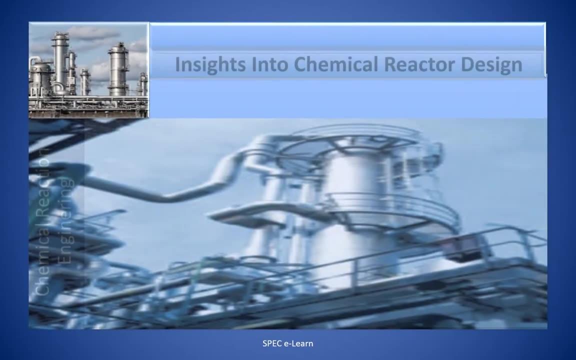 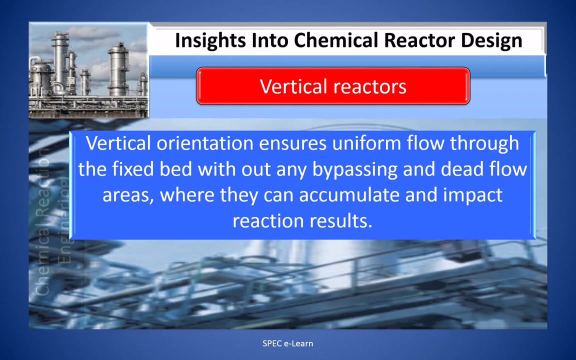 Vertical reactors is usually the choice when it comes to selecting the reactor type. Most of the industrial reactors in fertilizer and petrochemical industries are vertical reactors. Vertical orientation ensures uniform flow through the Fickbert without any bypassing and dead flow spots where they can accumulate and impact the reaction results. 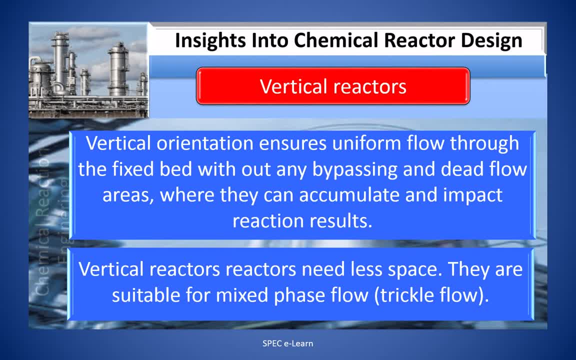 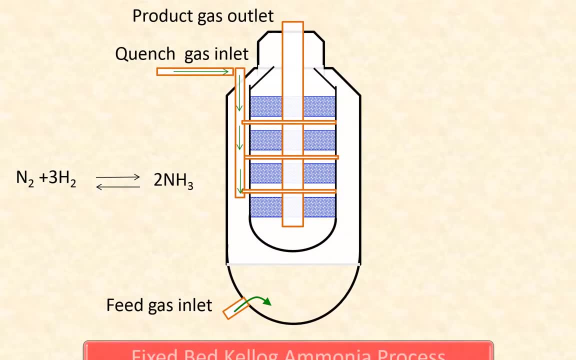 Vertical reactors need less space. They are suitable for mixed phase flow like trickle flow. The Fickbert catalog ammonia synthesis process is illustrated in this figure. It is illustrated in this figure is a vertical reactor, A fixed-bed catalog ammonia synthesis process. This is a four-bed catalytic process with a down flow. 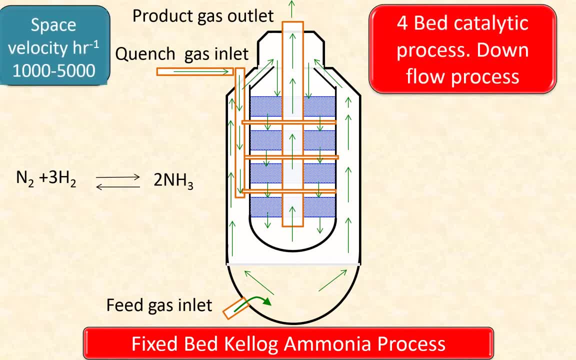 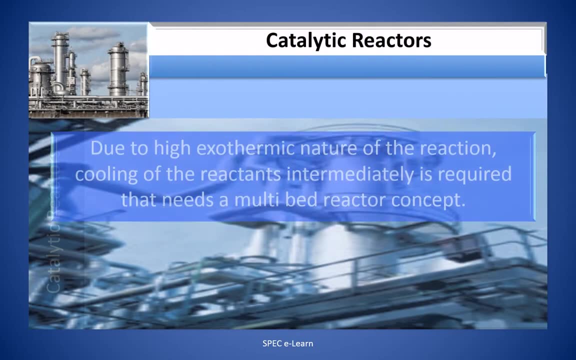 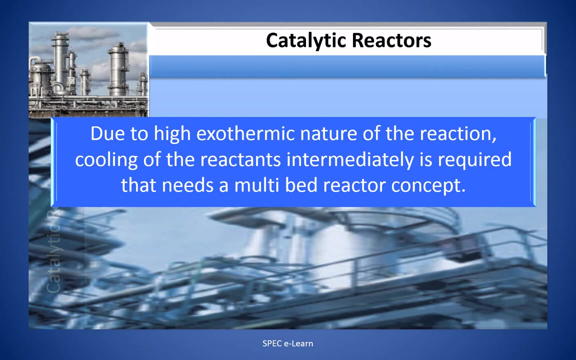 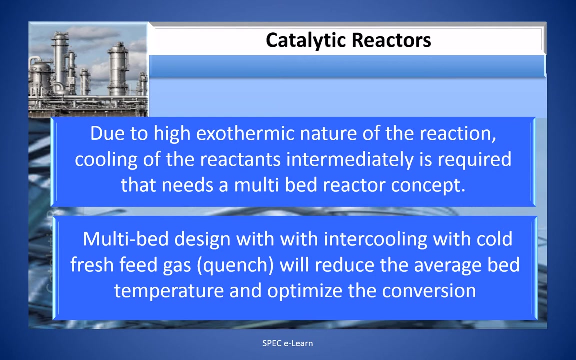 This is the Fickbert catalog ammonia synthesis process. Due to exothermic nature of the reaction, cooling of the reactants intermediately is required. that needs a multi-butt reactor concept. Multi-butt design with intercooling with cold fresh feed gas or quench will reduce average. 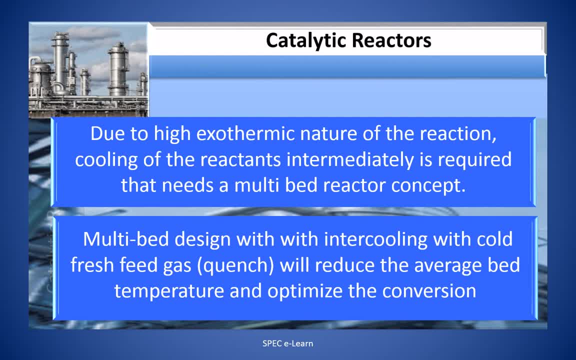 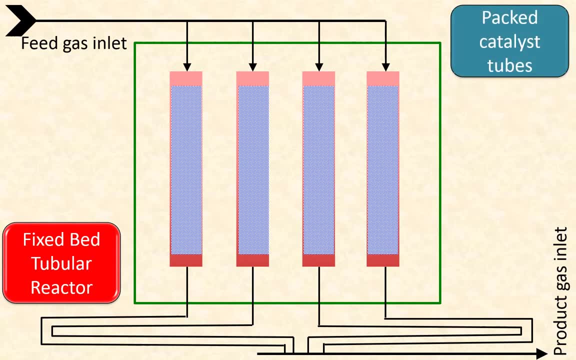 bit temperature and optimize conversion. Another vertically fixed bit reactor technology is tubular reactor. The engineering approach of this reactor technology is different from the one we just discussed in that it is endothermic reaction. Reaction is favored by high temperature. As the reaction proceeds and the fluid flowing down the reactor, the temperature drops. 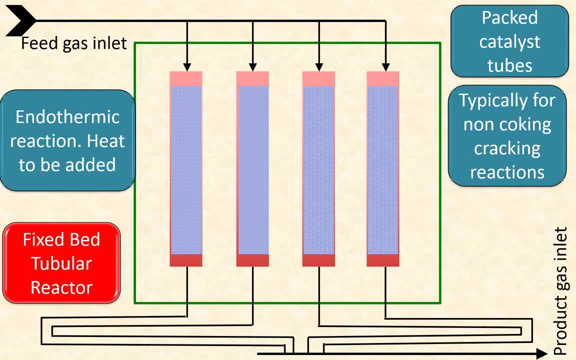 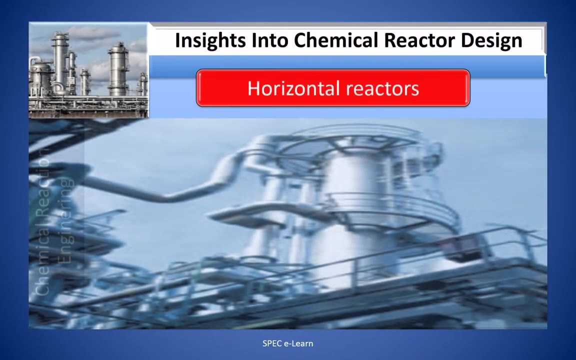 Hence heat needs to be added. A vertical row of tubes are placed in a furnace and heat is supplied by firing. Usually it is downflow reactor. The number of tubes, tube diameter, the tube length are the design parameters. Horizontal reactors are wide but relatively shallow. 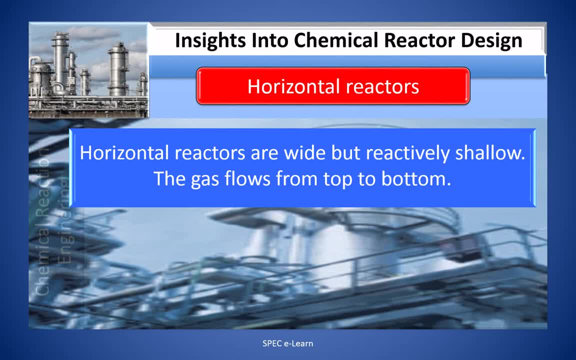 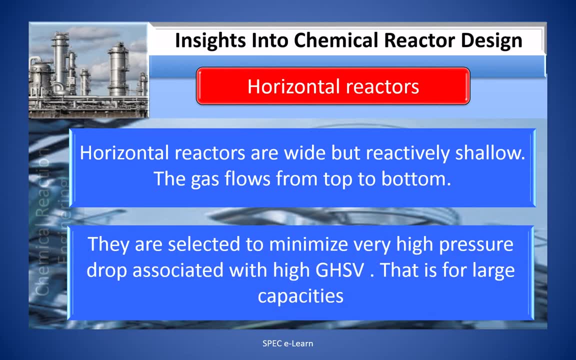 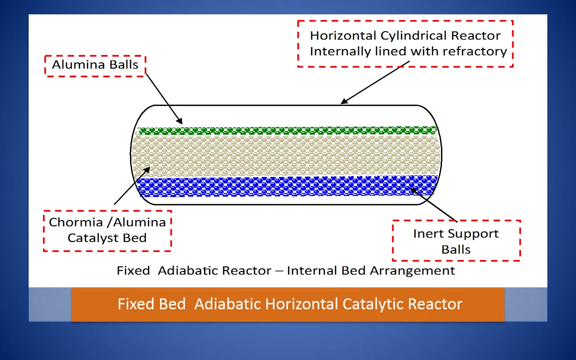 The gas flows down from top to bottom. They are selected to minimize very high pressure drop associated with high GHSV, that is, for large capacities. Illustrated in this figure is a fixed-bed adiabatic horizontal catalytic reactor, internally refractive line. 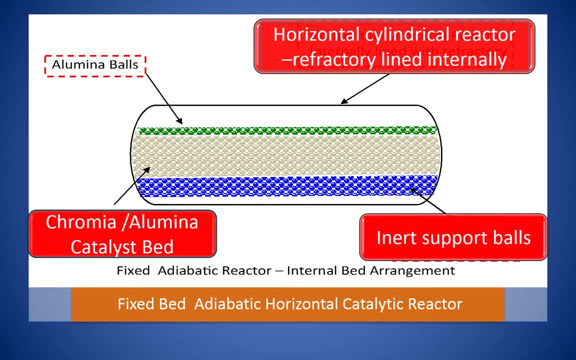 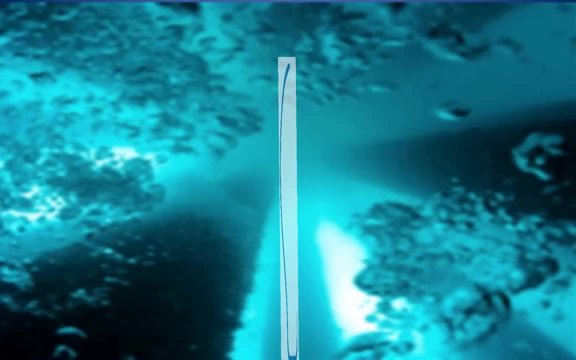 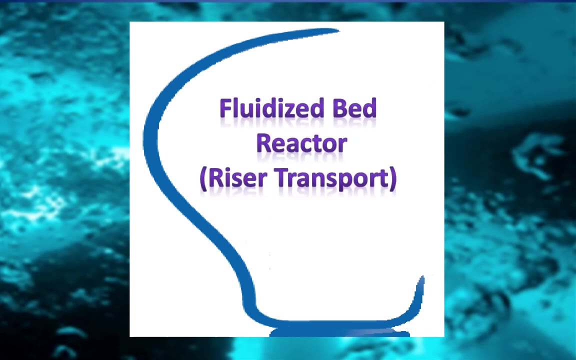 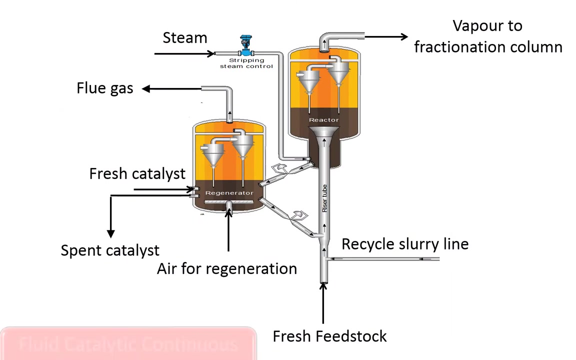 And externally insulated. The next important reactor technology is fluidized bed reactor riser transport. The figure shown here is a fluid catetate cracking unit. FCC units are widely used in refineries to produce higher value gasoline from gas oil. FCC units basically consist of two units. 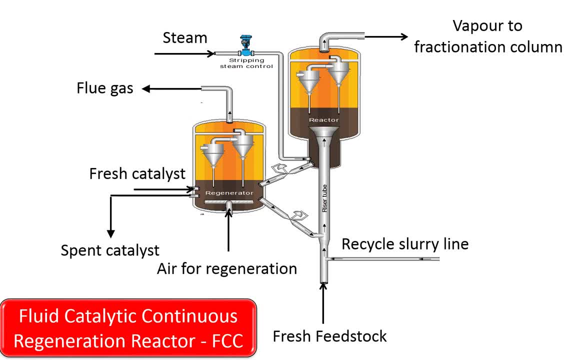 A reactor in which hot catalyst is brought into contact with feed, which is the gas oil, and a regenerator in which the coke deposited in the catalyst is banned off for regenerating the catalyst. The riser is an important part of the FCC. The conversion of heavy petroleum fraction occurs in the riser reactor, which is a long 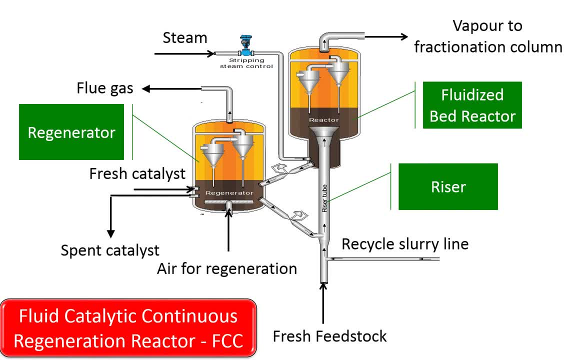 tube length of approximately 30 to 40 meters with proportionately small diameter, roughly 0.8 to 1.2 meters. After complete vaporization of the hydrocarbon feed, the two phases- solid catalyst phase and vapor phase, which is the hydrocarbon and steam- are left in the riser. 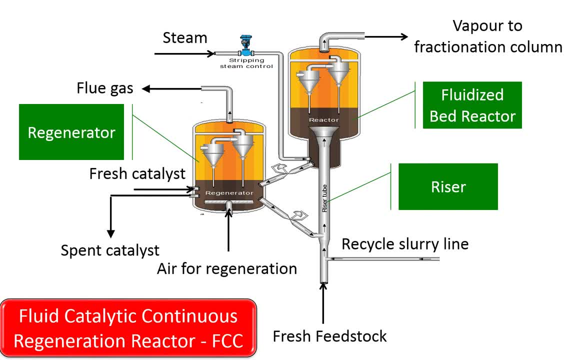 Catalytic reactions occur in the vapor phase. The decrease of density of the gas phase Due to cracking and the expanding volume to the vapor that are generated are the main driving force that is increasing velocity to carry the catalyst of the riser Catalyst and products are quickly separated in the reactor. 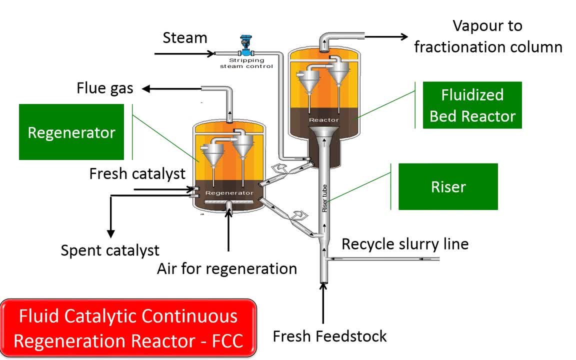 The product leaves the reactor at the top, The separated catalyst is drawn to a regeneration unit where it is contacted with hot air to ban off the coke And the catalyst gets regenerated. The regenerated catalyst is circulated back to the reactor again with a small amount of 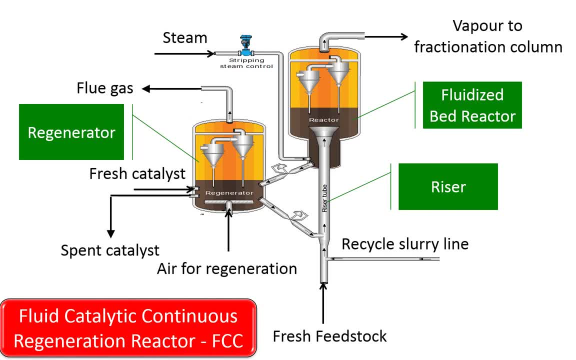 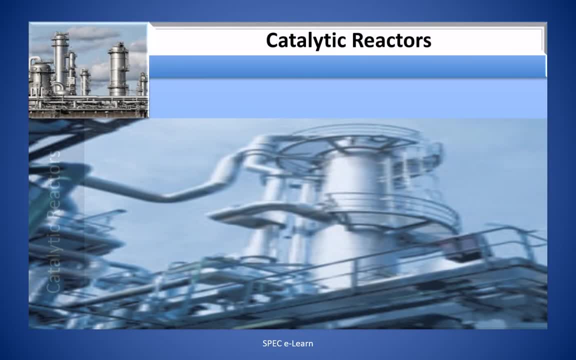 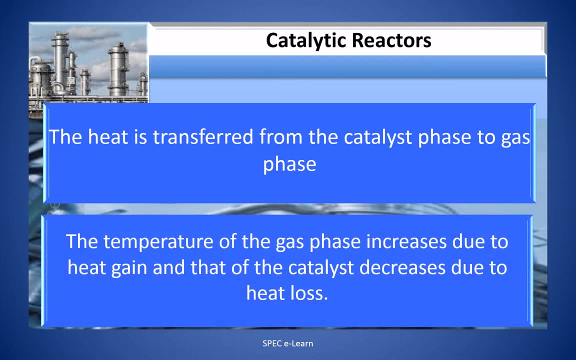 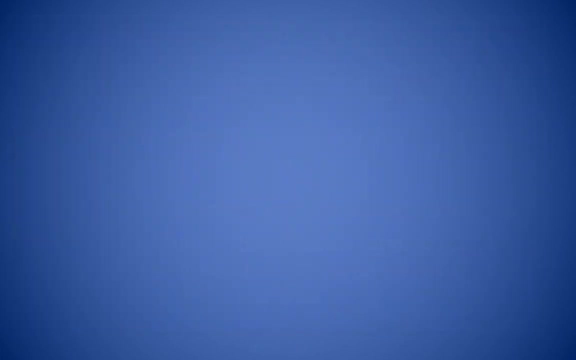 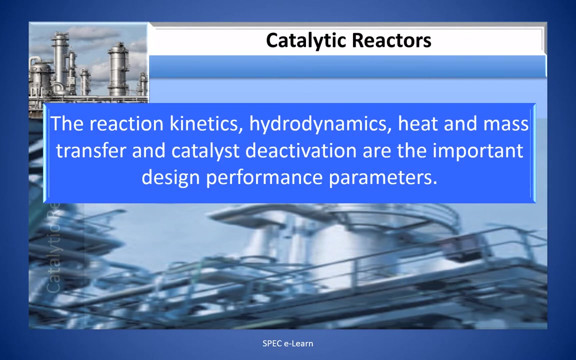 fresh catalyst. The heat is transferred from the catalyst phase to the gas phase. Temperature of the gas phase increases due to the heat gain And the catalyst decreases due to the heat loss. The reaction kinetics: hydrodynamics, heat and mass transfer and catalyst deactivation. 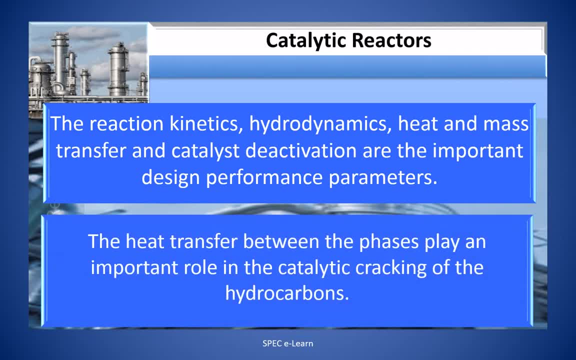 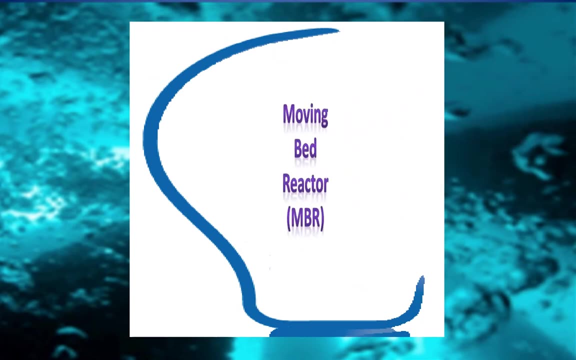 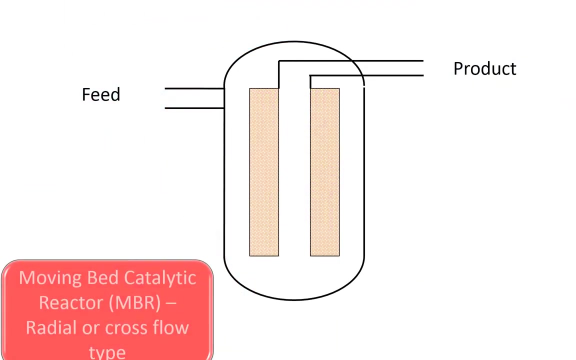 are the important design performance parameters. The heat transfer between the phases play an important role in the catalytic cracking of the hydrocarbons. Another widely used reactor technology is a moving bed reactor. Shown in this figure is a moving bed catalytic reactor. 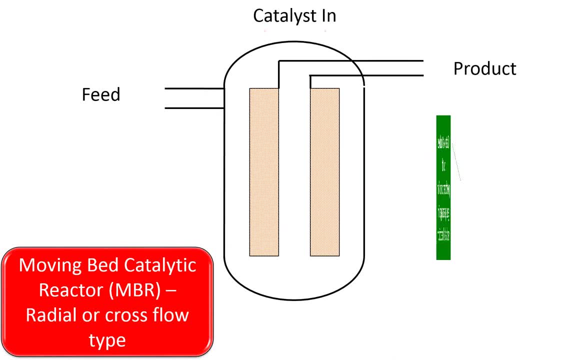 Note that the rows of perforated tubes are installed vertically in the reactor. The catalyst particles enter at the top end of the tube and moves down, while the gas enters radially through the perforations in the tube. After reacting with the catalyst, the gaseous products of reaction moves out of the tube. 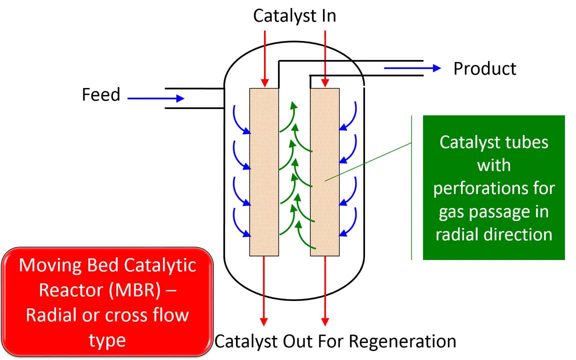 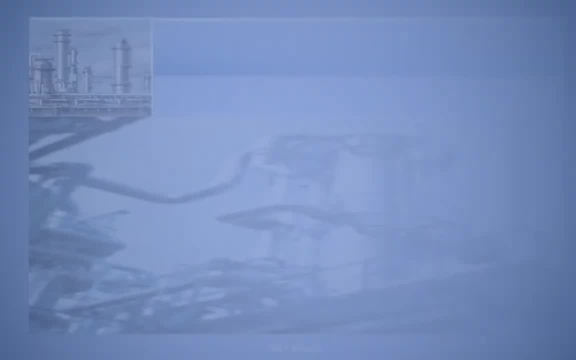 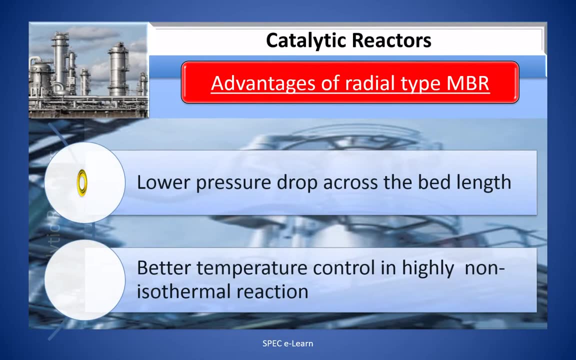 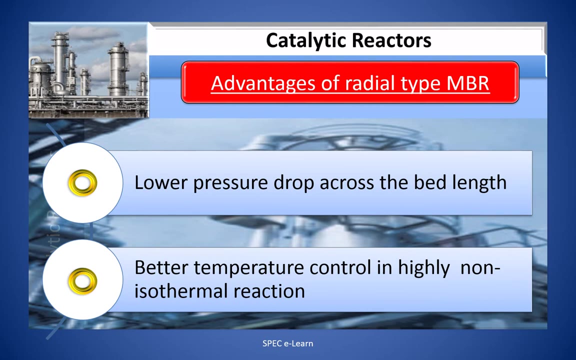 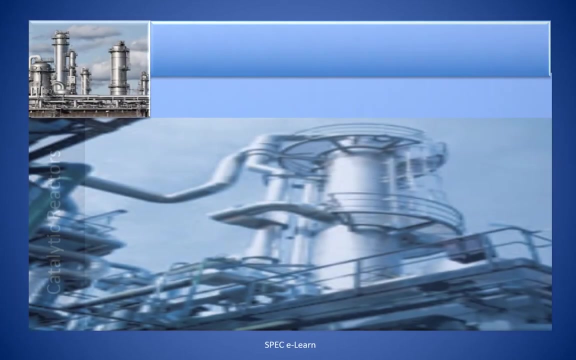 and leaves the reactor at the top. The advantages of radial tape in B-R is low pressure drop across bed length and better temperature control in higher temperatures. It is also a reliable and efficient reactor. We can use it for various purpose in highly non-isothermal reaction. moving bed reactor can also have other flow arrangements. 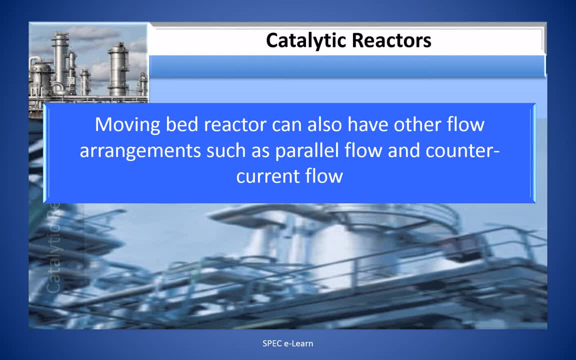 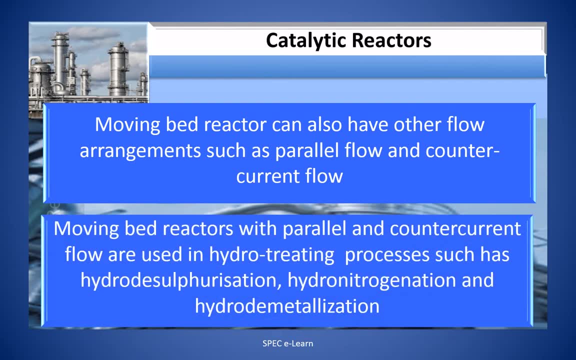 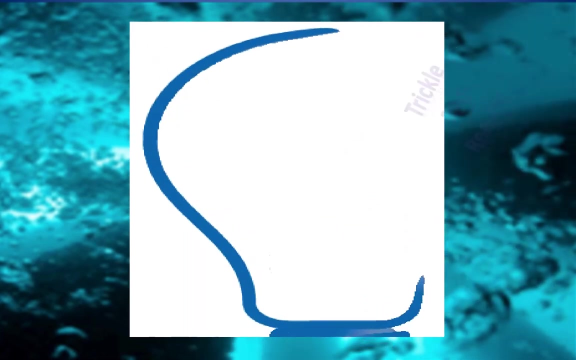 such as parallel flow and counter current flow moving. but reactors with parallel and counter current flow are used in hydro treating processes such as hydro desulphurization, hydro nitrogenization and hydro demetallization. another widely used type of reactor is a trickle bed reactor. 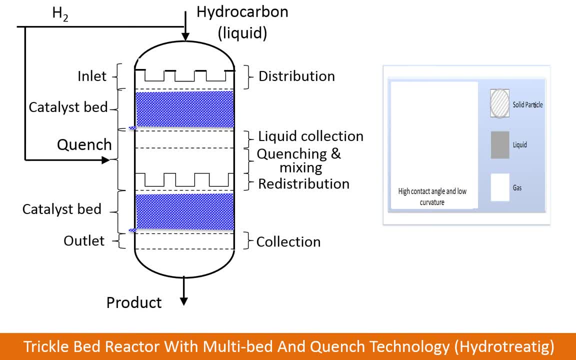 shown in this figure is a trickle bed reactor used in the hydrotreating of petroleum products. the reactor is of fixed bed type. like in packed mass transfer column, the liquid and gas mixture is distributed over the bed. the liquid tickles down the bed while the reaction is in progress. 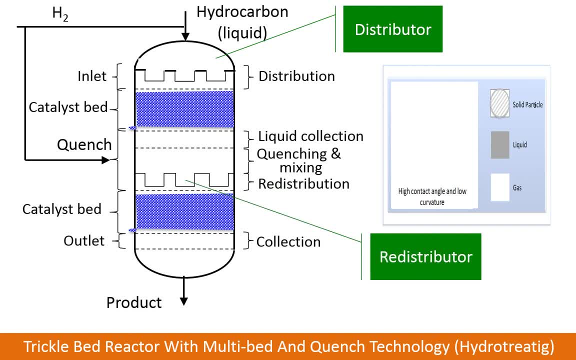 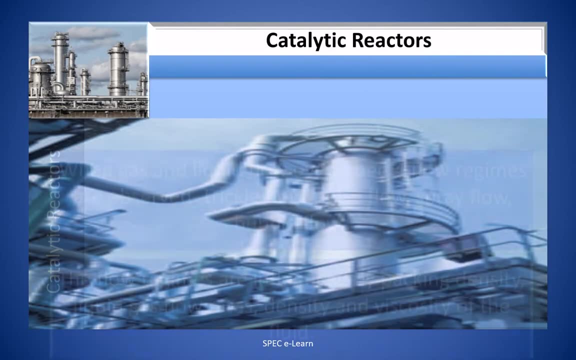 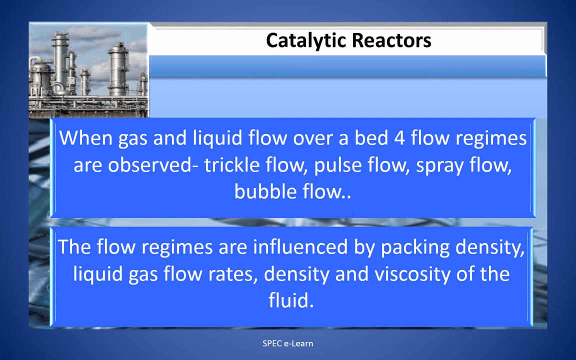 the catalyst points the surface for reaction between the gas and the liquid. due to exothermic reaction, multi-bed quenching technology is required. we'll see that. before we move to the next type of reactor technology, let me throw some light on the hydrodynamics of the flow regimes when a liquid and gas flow over a solid surface. 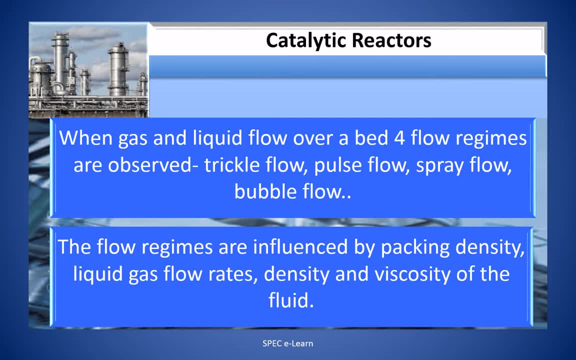 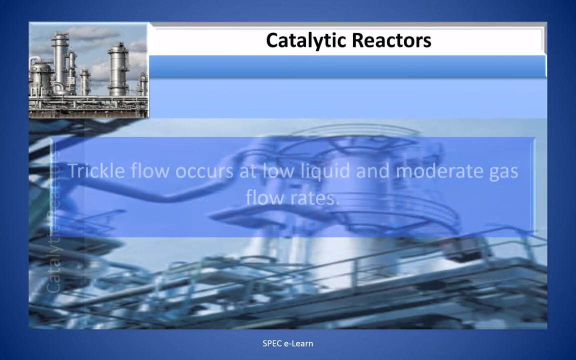 when gas and liquid flow over a bed, four flow regimes are usually observed: trickle flow, pulse flow, spray flow and bubble flow. The flow regimes are influenced by the packing density, liquid gas flow rates, density and viscosity of the fluid. Trickle flow occurs at low liquid and moderate gas flow rates. 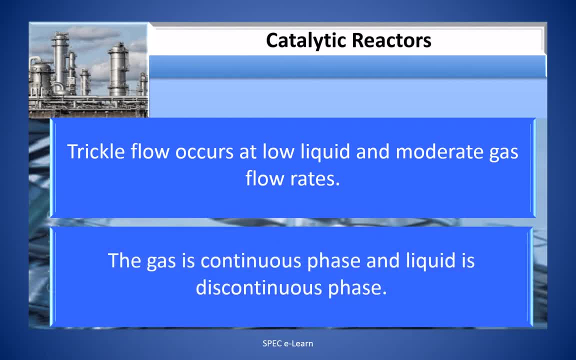 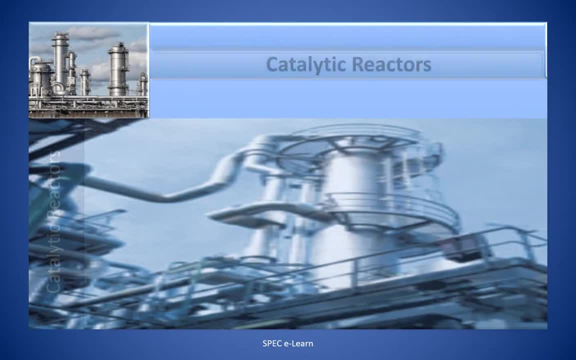 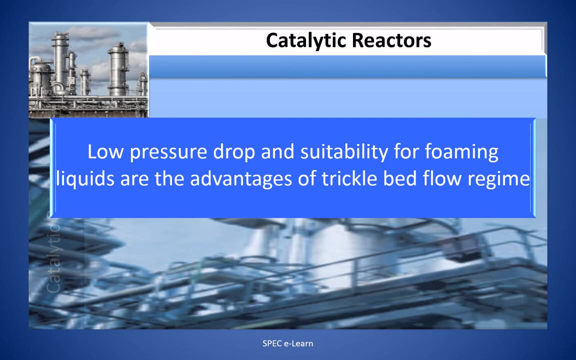 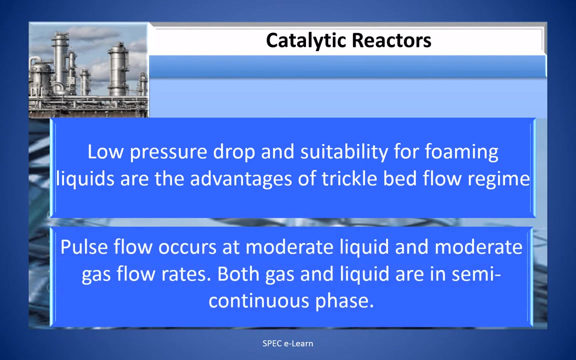 The gas is continuous phase and liquid is discontinuous phase. Low pressure drop and suitability for formal liquids are the advantages of trickle bed flow regime. Pulse flow occurs at moderate liquid and moderate gas flow rates. Both gas and liquid are in semi-continuous phase. 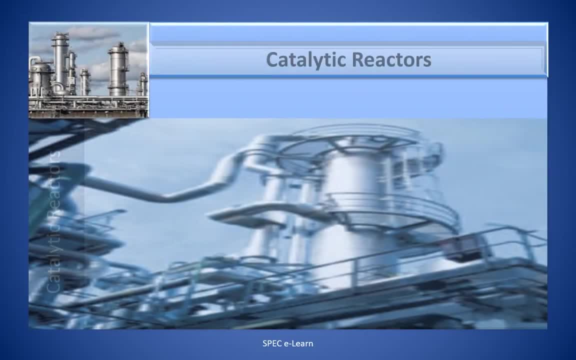 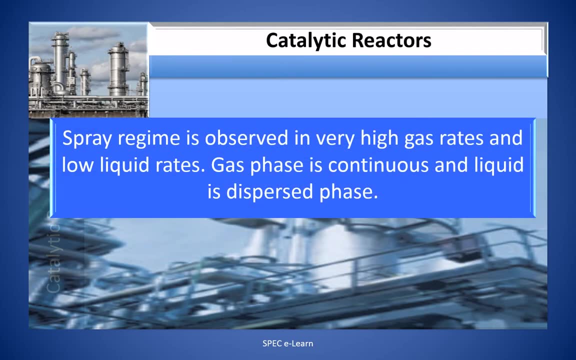 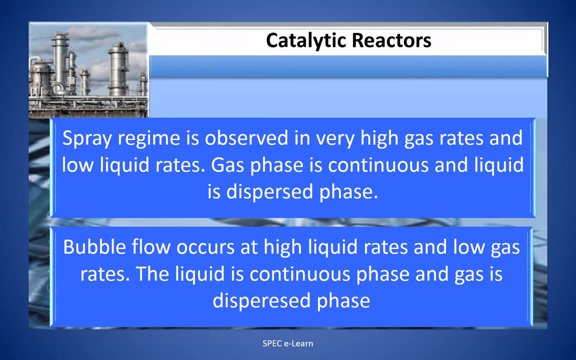 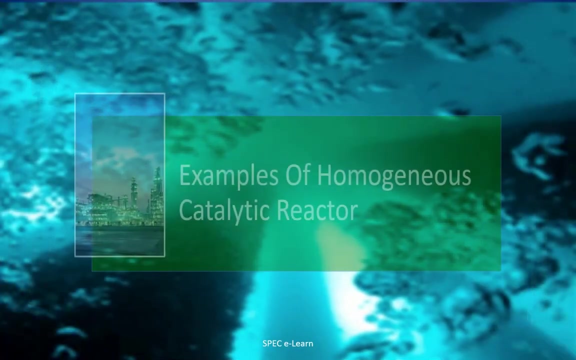 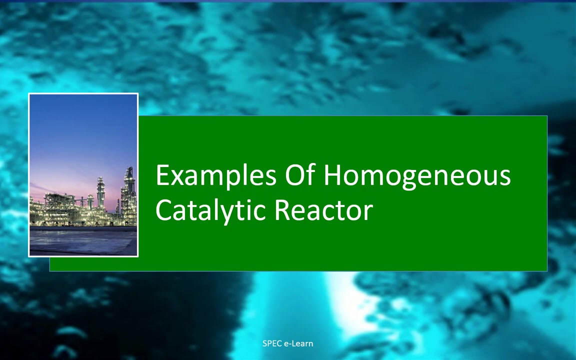 Spare regime is observed in very high gas rates and liquid rates. Gas phase is continuous and liquid is dispersed phase. Bubble flow occurs at high liquid rates and low gas rates. The liquid is continuous phase and the gas is dispersed phase. Having seen the different types of heterogeneous reactor, we will move on to see an example of homogeneous catalytic reactor. 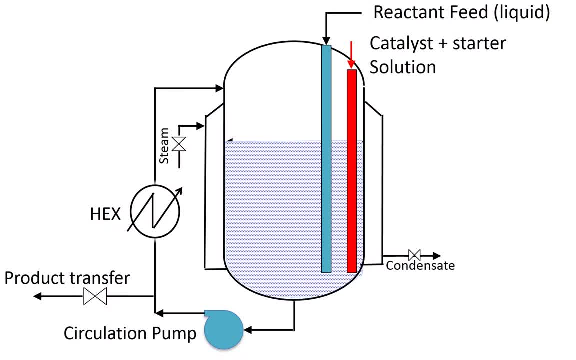 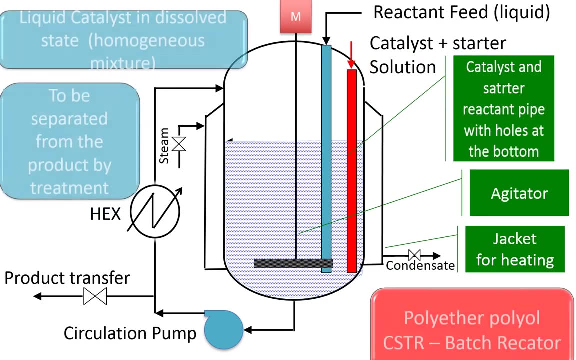 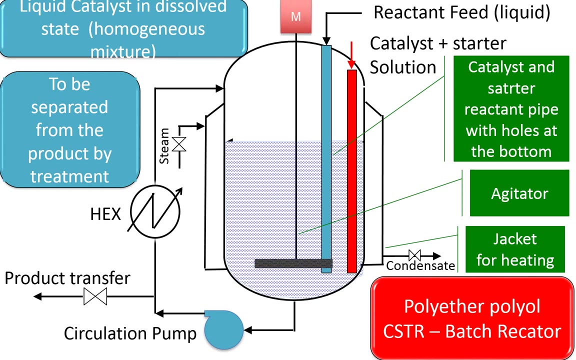 Shown in this figure is a batch homogeneous catalytic reactor. Catalyst with some starting reactant is fed initially into the reactor. The second reactant in the liquid phase is continuously fed and agitation is maintained during the reaction. The reaction product is circulated by a pump externally through an exchanger to remove the heat of reaction continuously. 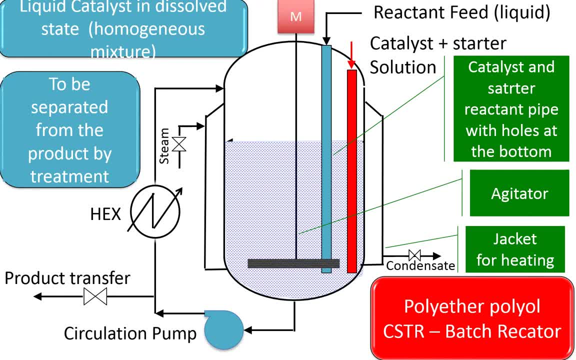 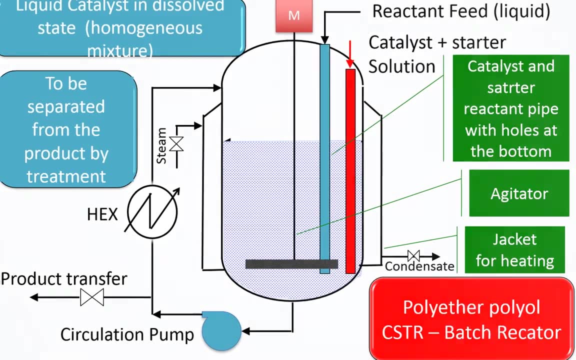 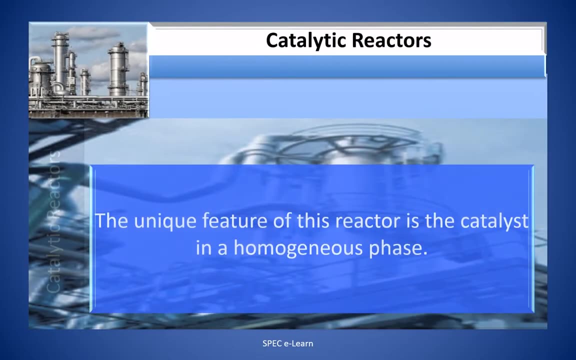 When the required batch size is achieved, the feed addition is terminated. After that, the product containing the catalyst is discharged from the reactor to another processing vessel Where the catalyst is separated. The unique feature of this reactor is the catalyst is in a homogeneous phase. 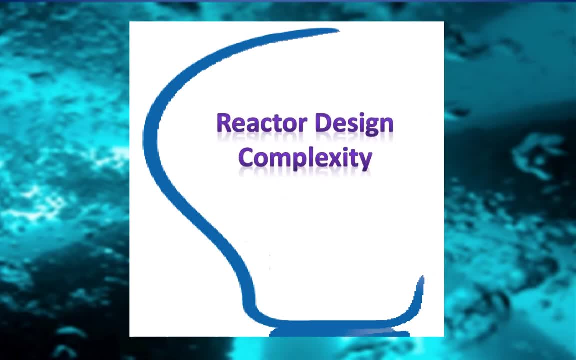 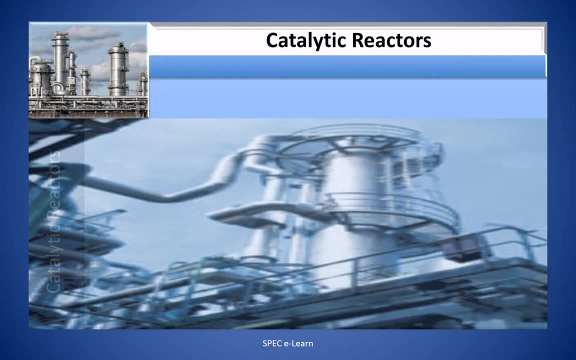 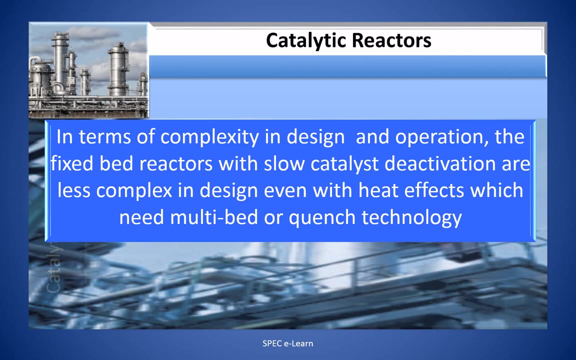 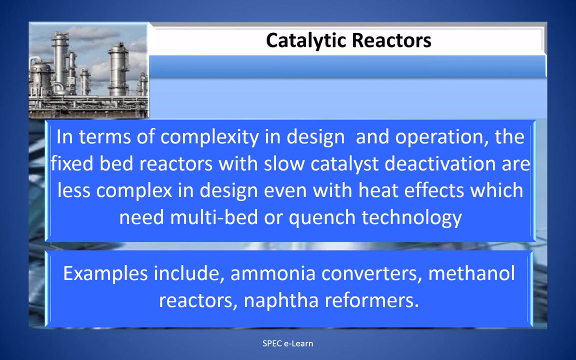 Reactor design complexity. In terms of complexity in design and operation. the fixed-bed reactors with slow catalyst deactivation are less complex in design, even with heat effects with multi-bed or quench technology. Examples include ammonia converters, methanol reactors and naphtha reformers. 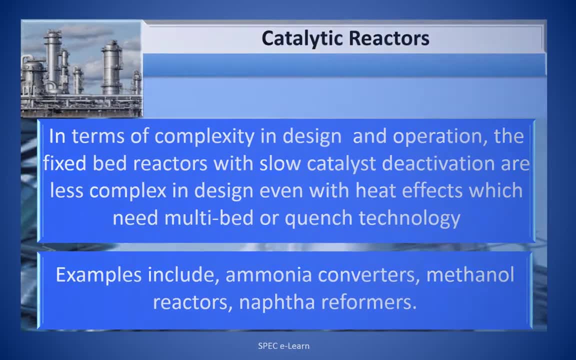 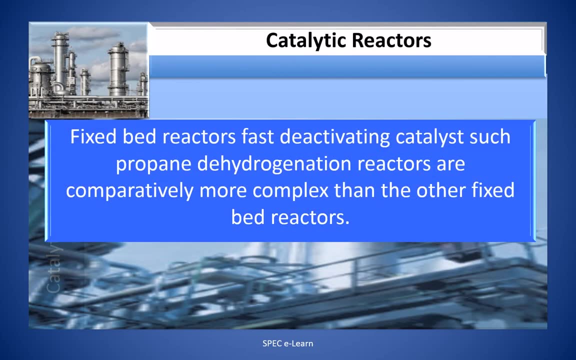 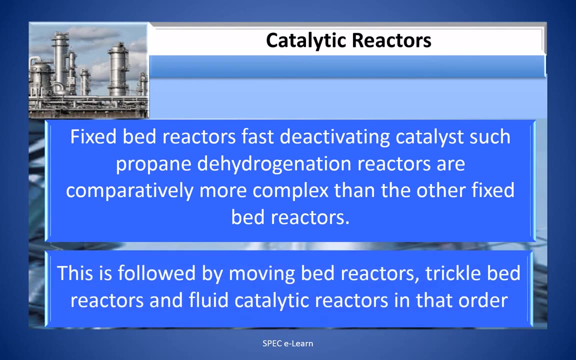 Fixed-bed reactors with fast deactivating catalysts, such as propane decardigination reactors, are comparatively more complex than the other fixed-bed reactors mentioned above. This is followed by moving-bed reactors, trickle-bed reactors and fluid catalytic reactors, in that order of complexity. 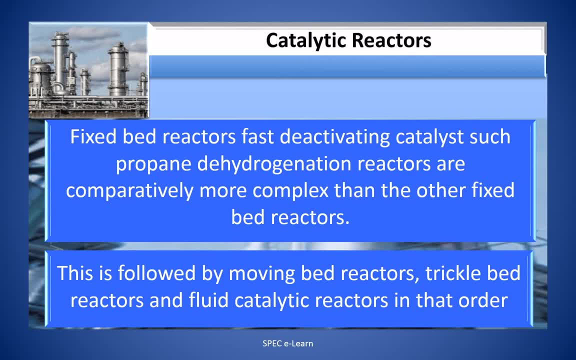 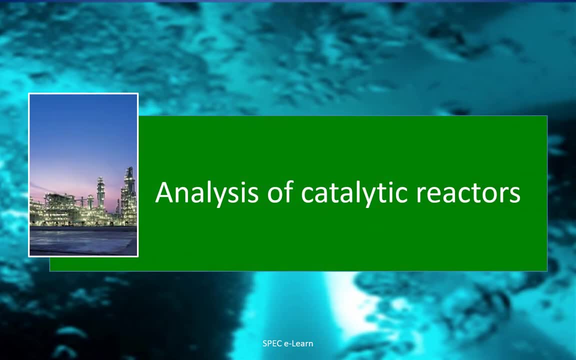 This is followed by moving-bed reactors, trickle-bed reactors and fluid catalytic reactors, in that order of complexity. So far, we had focused our attention on the engineering approaches for designing and selection of catalytic reactors. We will shift our focus to the analysis of catalytic reactors. 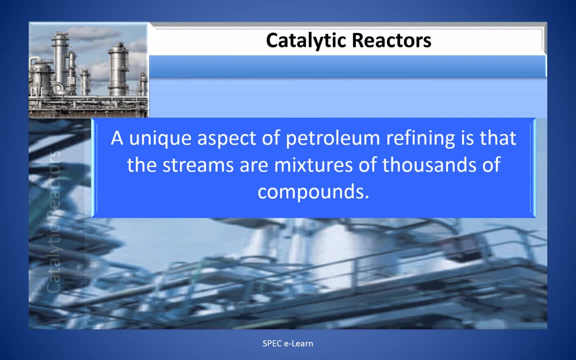 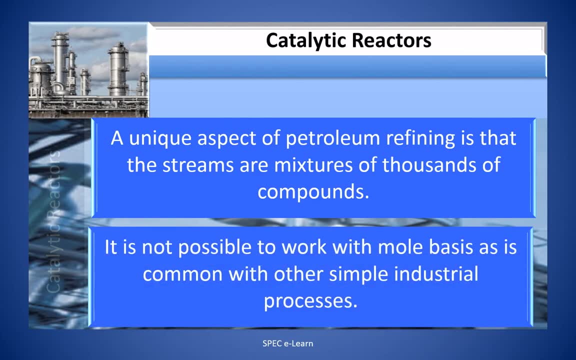 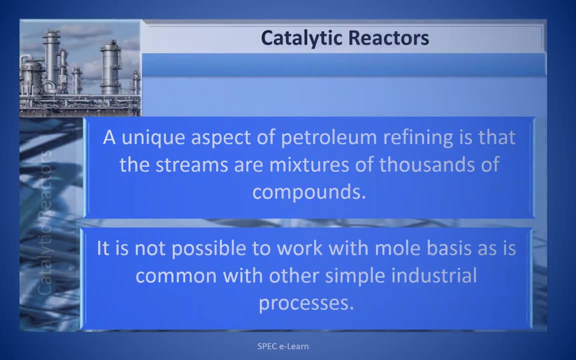 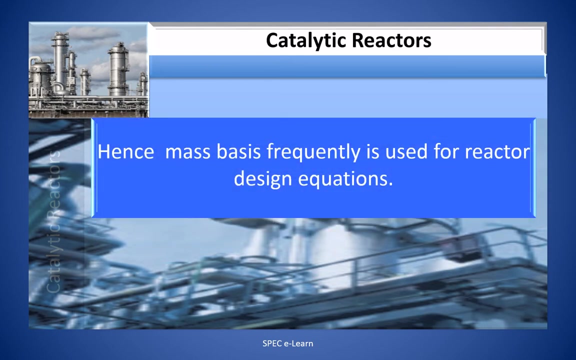 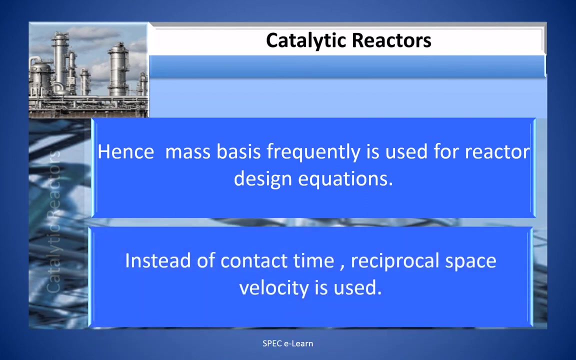 A unique aspect of petroleum refining is that the streams are mixers of thousands of compounds. It is not possible to work with mole bases, as is common with other simple industrial processes. Hence mass basis is frequently used for reactor design equations. Instead of contact time, reciprocal space velocity is used. 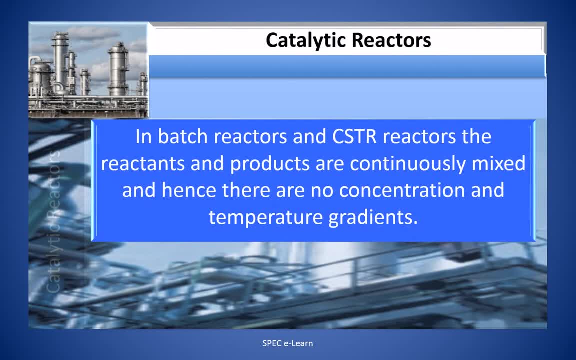 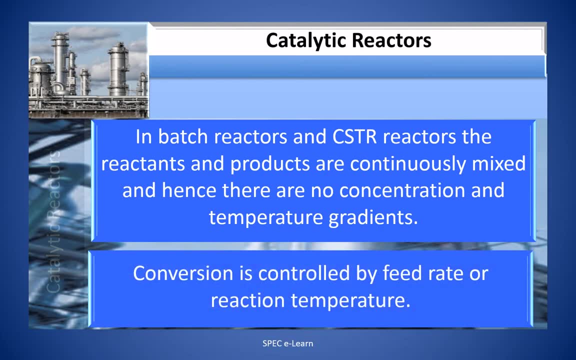 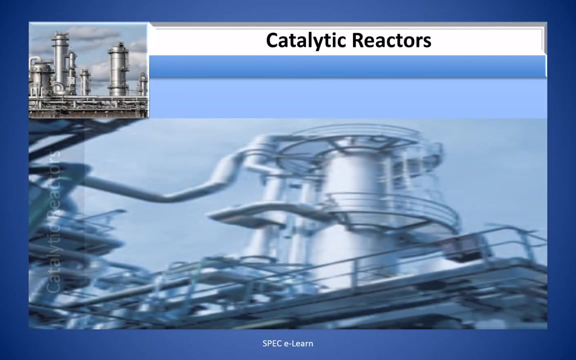 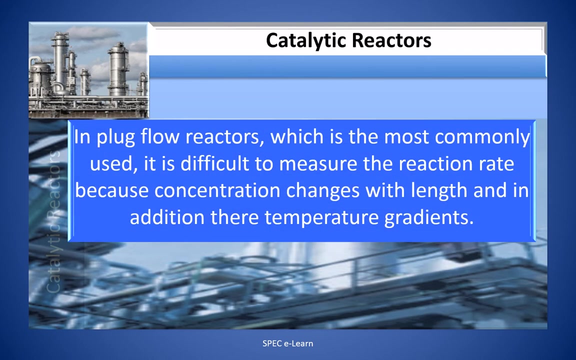 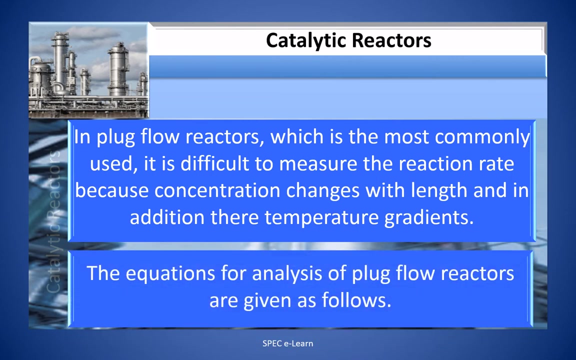 In batch reactors and CSTR reactors, the reactants and the products are continuously mixed and hence there are no concentration and temperature gradients. Conversion is controlled by the feed rate or the reaction temperature. In contrast, in plug-flow reactors, which is the most commonly used, it is difficult to measure the reaction rate because the concentration changes with the length and, in addition, there are temperature gradients. 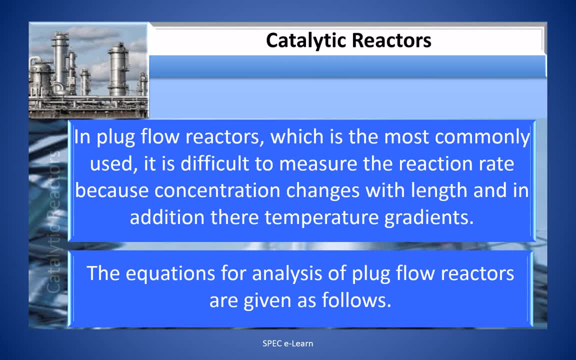 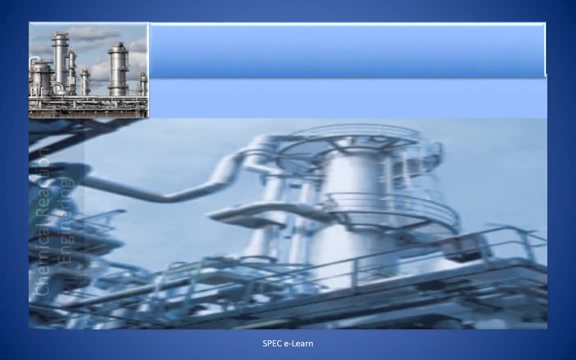 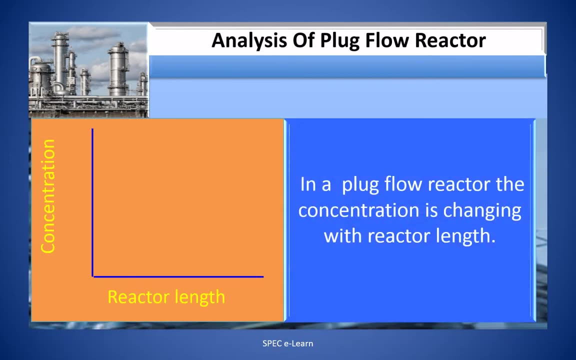 The equations for analysis of plug-flow reactors are given as follows. As illustrated in the figure on the left, in a plug-flow reactor the concentration is changing with the reactor length Note. from the initial concentration, the Ca note, it decreases to Ca at the end of the reactor. 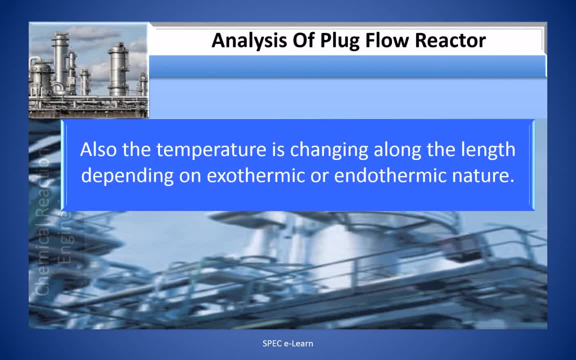 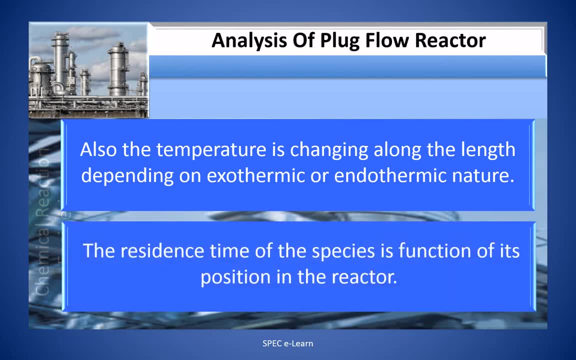 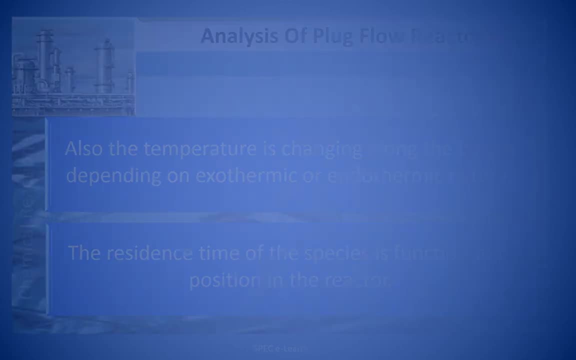 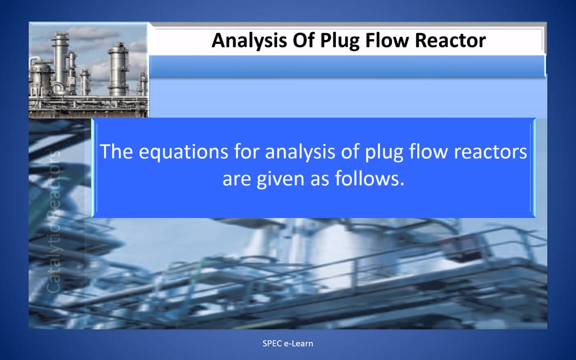 Also, the temperature is changing along the length, depending on whether the reaction is exothermic or endothermic in nature. The residence time of the species is a function of its position in the reactor. Shown here is the equation for analysis of plug-flow reactor. 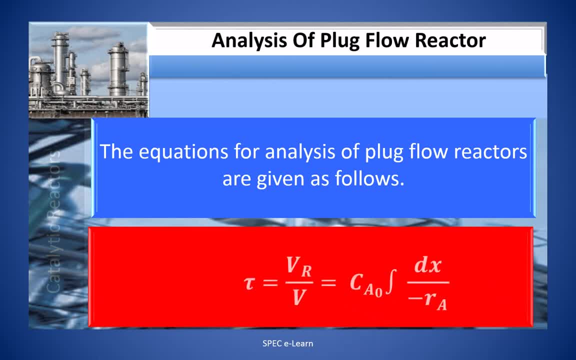 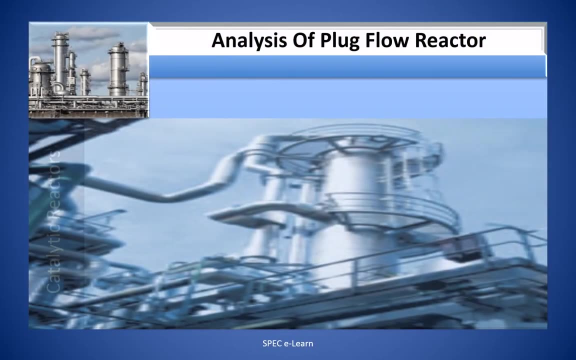 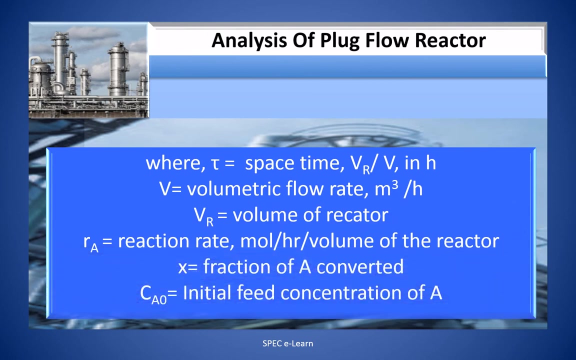 Tau is equal to Vr by V, which is equal to Ca note integral of dx by minus Ra, Where tau is the space time in hours. V is the volumetric flow rate in meter cube per hour. Vr is the volume of the reactor. 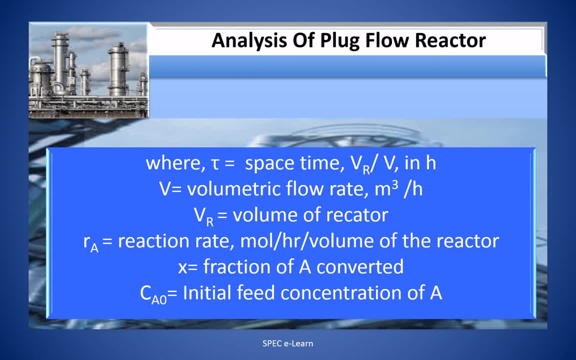 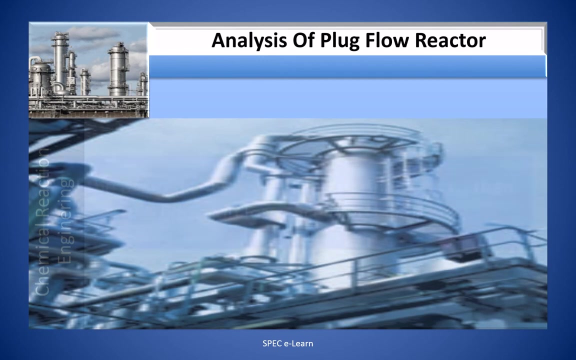 Ra is the reaction rate. Tau is the reaction rate in moles per hour per unit volume of the reactor. X is a fraction of A converted Ca. note is the feed concentration of A at the reactor inlet If the desired conversion of component A is Xaf. 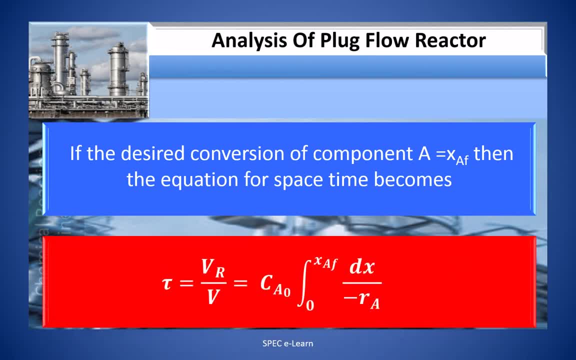 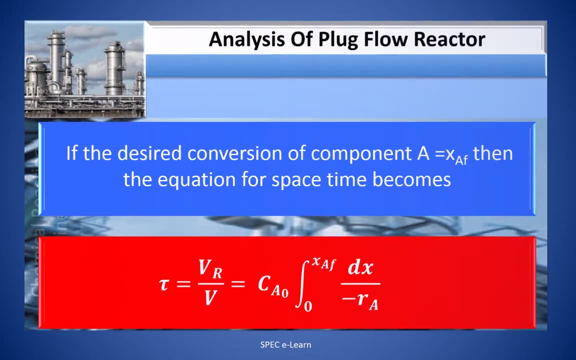 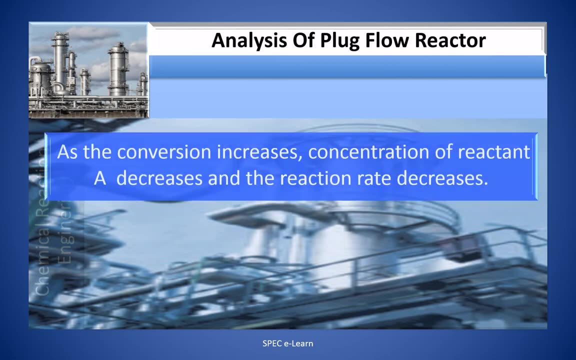 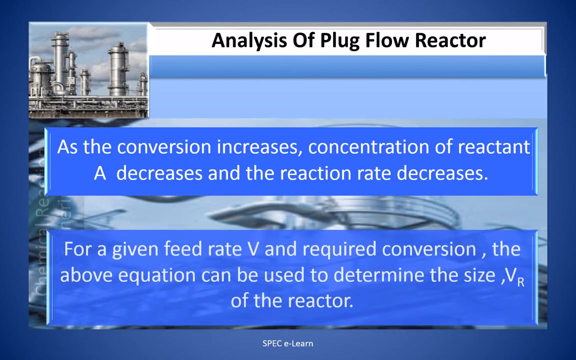 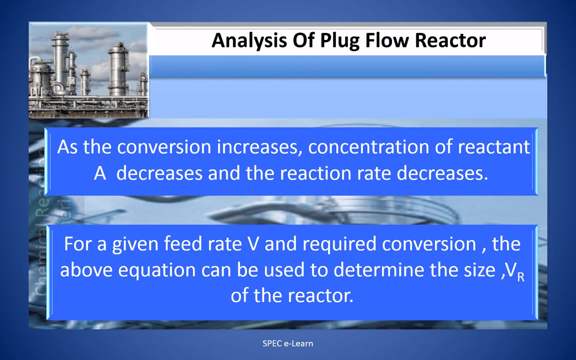 then the space time is obtained by integrating the above equation from 0 to Xaf. As the conversion increases, the concentration of reactant A decreases and the reaction rate decreases. For a given feed rate, V and required conversion, the above equation can be used to determine the size Vr of the reactor. 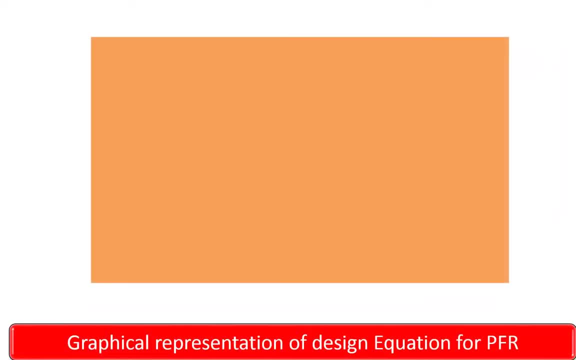 So the problem is to determine the size in which the area is under the curve. The area under the curve is tau by Ca naught. The area of the curve is tau by Ca0.. The area of the curve is tau by Ca0. 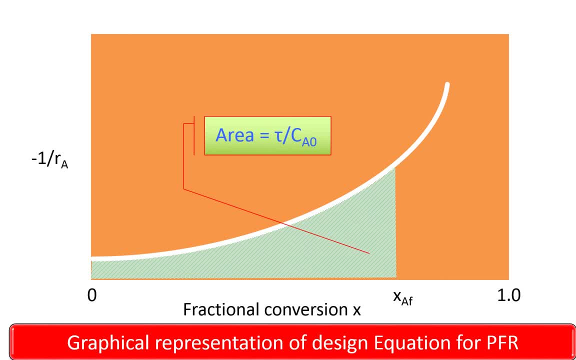 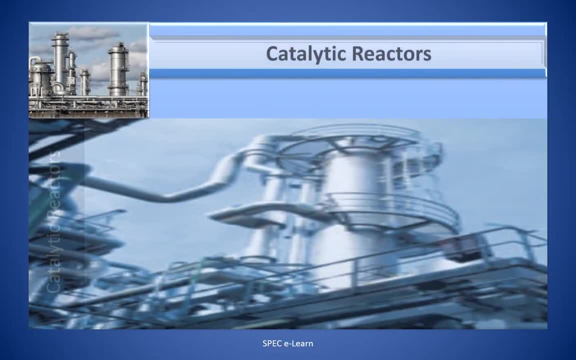 The area under the curve is tau by Ca0.. The area is under the curve is tau by Ca0.. Now let us discuss the plot of minus 1 by Ra. Now let us come to the plug flow catalytic reactors. The above equation for simple plug flow reactor can be used for sizing catalytic plug flow. 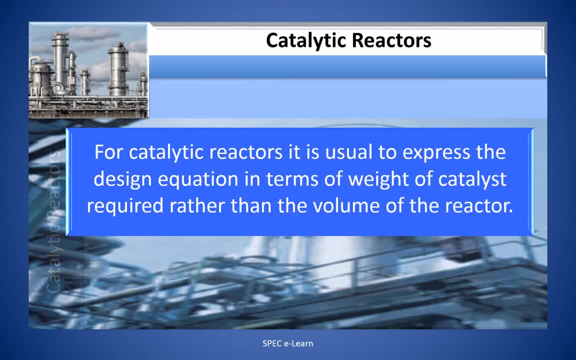 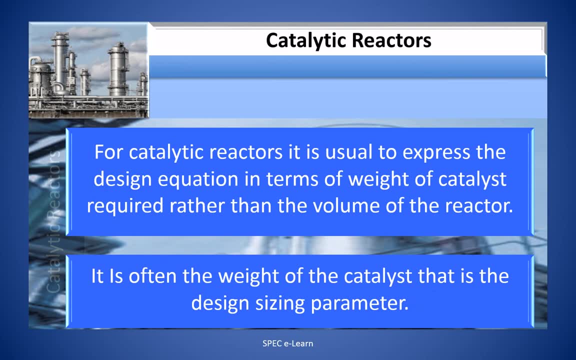 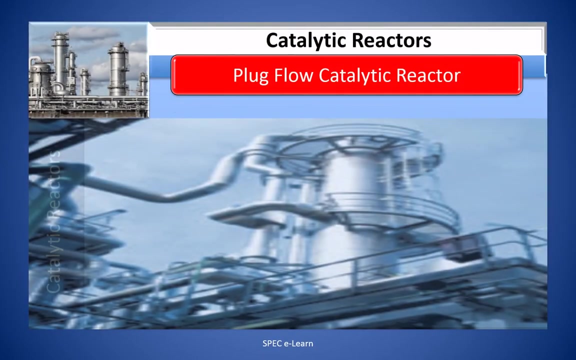 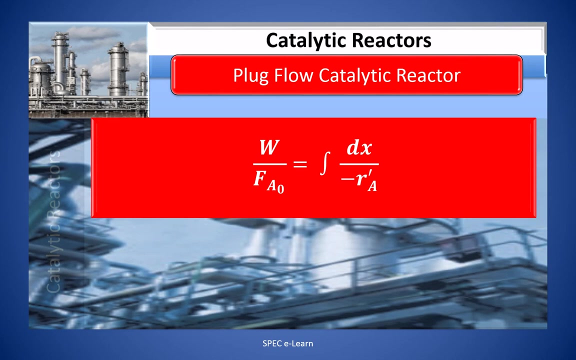 reactors. also For catalytic reactors it is usual to express the design equation in terms of the weight of catalyst required rather than the volume of the reactor. This often the weight of the catalyst that is the design sizing parameter. So the design equation for the catalytic plug flow reactor is: WFi0. equals integral of dx. 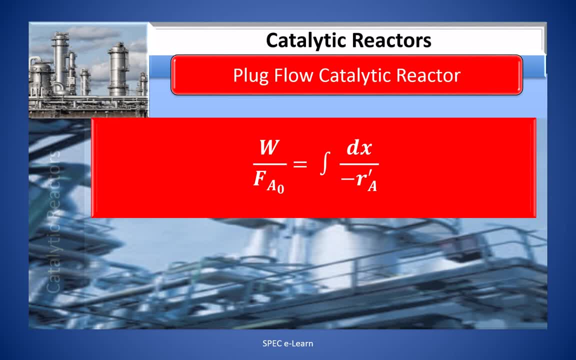 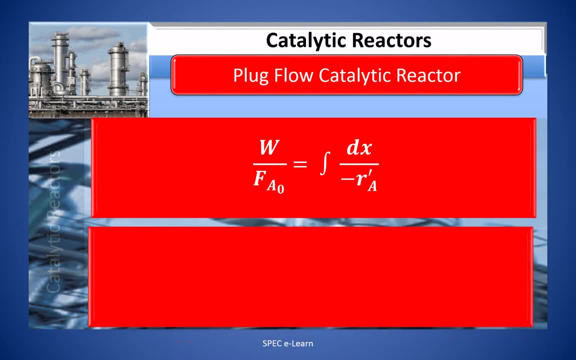 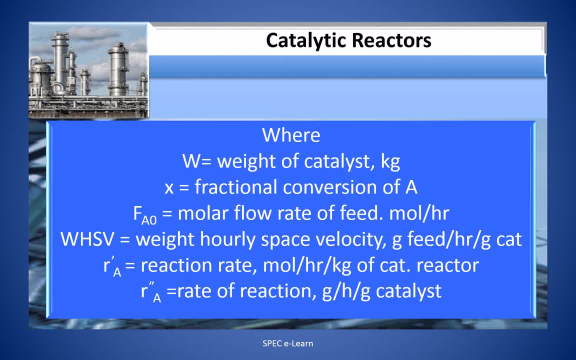 Where W is a weight of catalyst, x is a fractional conversion of a. FA0 is a molar flow rate of feed in moles per hour. WHSV is a weight over space velocity. It is a molar flow rate of Catalyst in grams per hour. 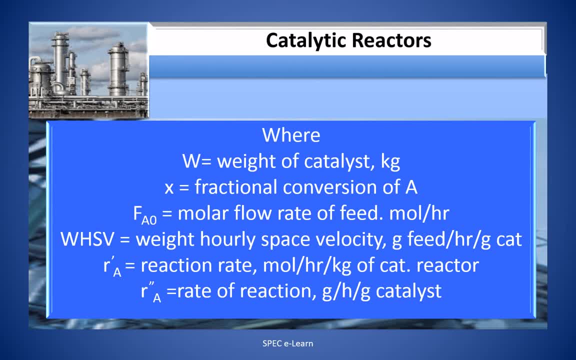 For catalytic Okho person. we understand Sirius as little less than shades per hour of degree energy. You, celebrity, can translate this parameter in post 65 degree yourself. But here you have to carry this thing further. for the further 치+, because we've already shown this parameter in previous sequences. 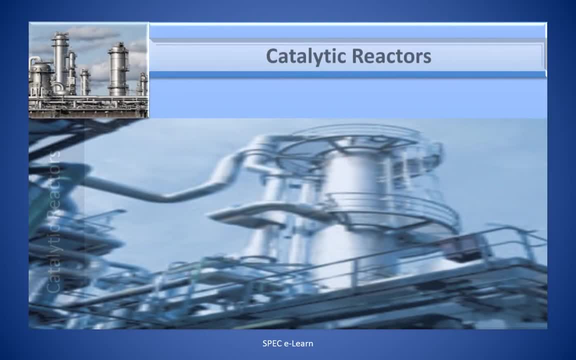 So. So today we weigh byitt and the down figure of UG And year UG in our local concentration divergence. We check number of days, measured of fertility and the times. so we will carry uOd. Then for the secondowner esteem, the constant Kelvin mass should not be more than 0.820.. 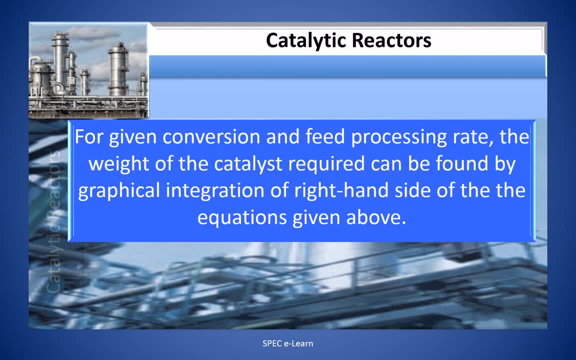 Therefore, by Morbih, we need to apply the coefficient of Gram followers per room per gram of catalyst rate. the weight of the catalyst required can be found out by graphical integration of the right hand side of the equation given above. A plot of –1 by rA can be made for. 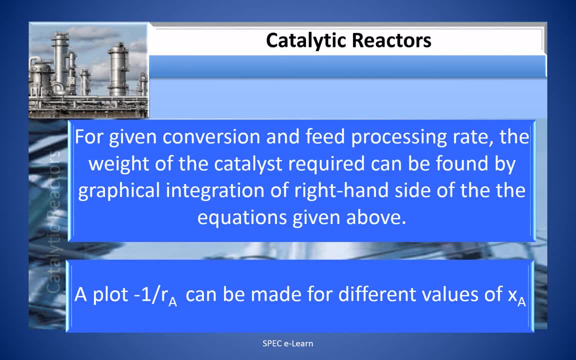 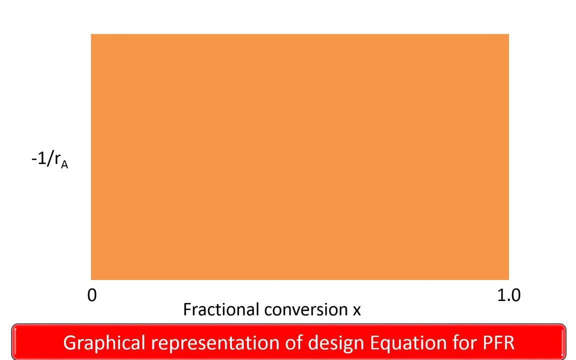 different values of xA. This is the plot of –1 by rA versus fractional conversion in a catalytic reactor. For a given conversion, the area under the graph can be found out. The area under the graph equals 1 by weight over the space velocity. It is also equal to the weight of catalyst divided. 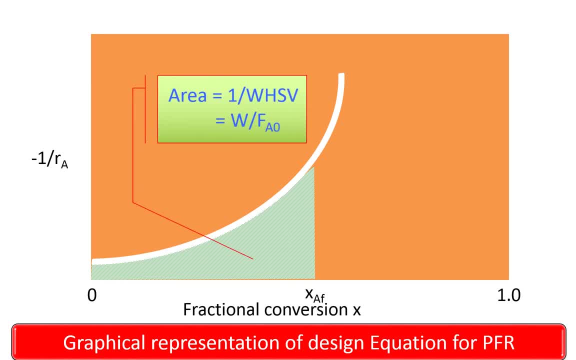 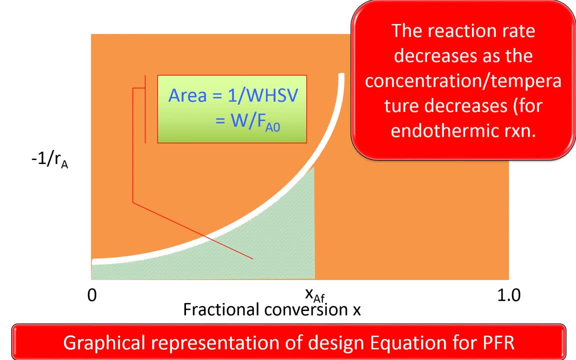 by the molar flow rate. The reaction rate decreases as the concentration decreases. And also for endothermic reaction, the reaction rate decreases as the temperature decreases. 1 by rA, the reciprocal of the reaction rate curve increases as the conversion x increases. 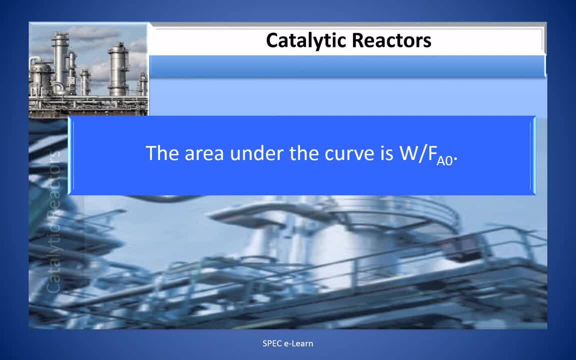 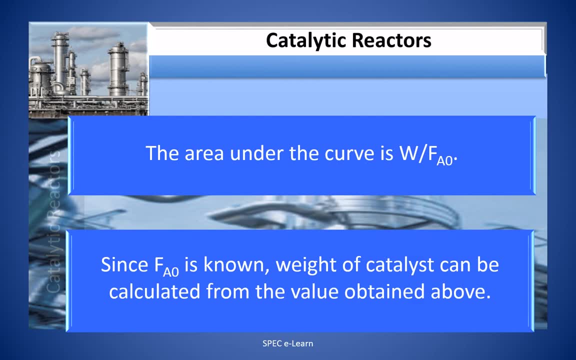 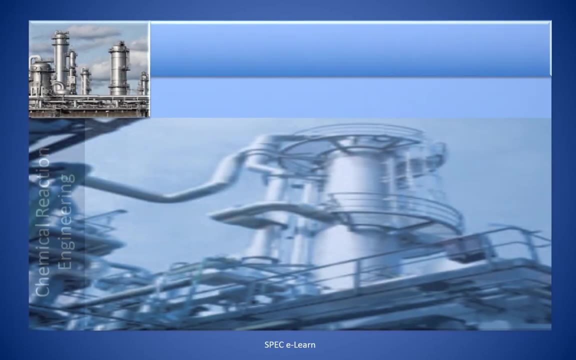 As we have seen in the figure, the area under the curve is WFA0 for a given conversion. Since FA0 is known, the weight of the catalyst can be calculated from the value obtained above. This is the end of this video. Please subscribe to our channel and get.